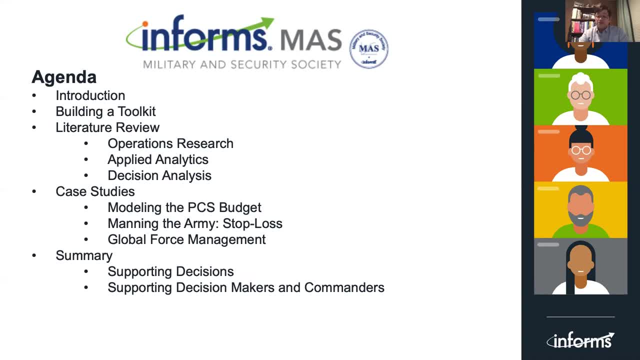 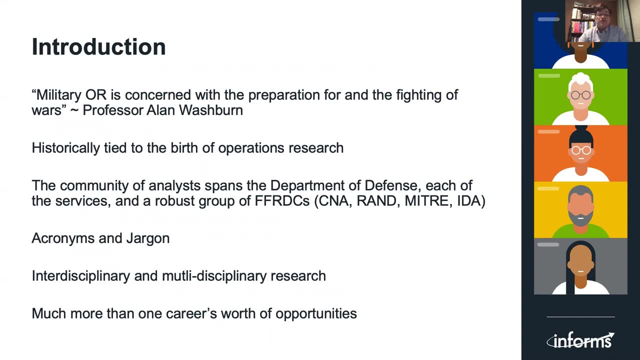 and commanders in our role as operations research analysts in the Department of Defense. Military operations research is concerned with the preparation for and fighting of war. This is a quote from Professor Alan Washburn in his chapter on military operations research within the Handbook of Public Sector OR. 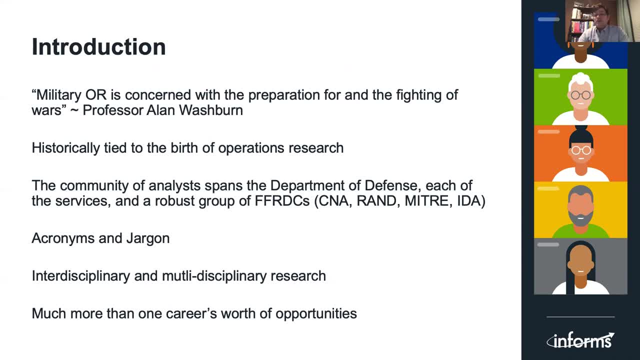 And one of the things that's interesting about military OR is that often we're working on edge cases. There is some really interesting problems. Often efficiency is not the objective function. Often you're trying to get the absolute best, The best of something, either the best armor, the longest shooting tank there are often 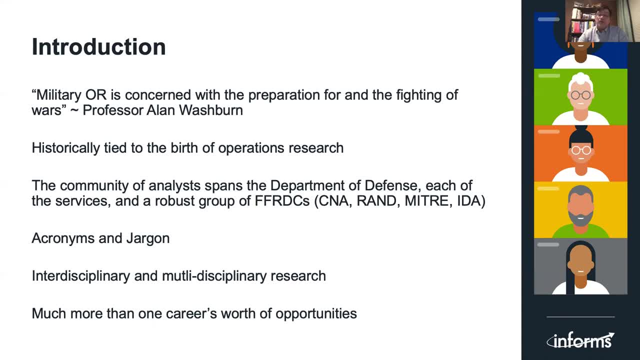 additional capability is actually a premium And historically, military operations research and operations research started as one in the same. The Second World War saw the birth of operations research. the Allies look to apply the means of the scientific method, the means of the physicists and mathematicians, and bring them together on to multi-disciplinary 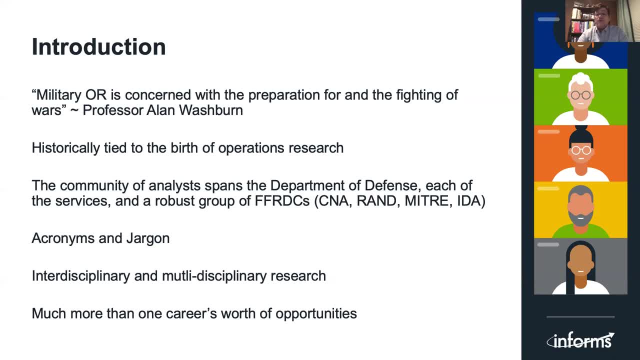 teams to try to solve problems that we'd never looked at before, And some of the things that came out of this early work- things like radar and search and detection theory- are some of the earliest successes in operations research. The community today of operations research analysts that focus. 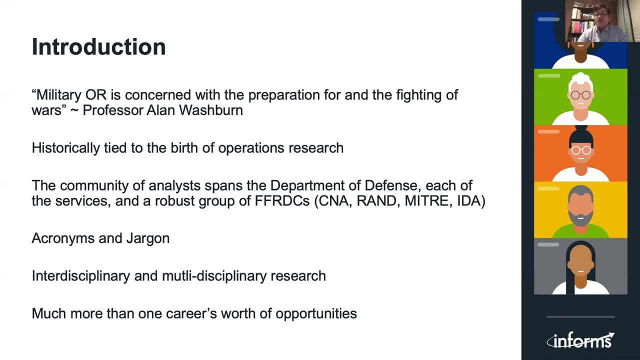 on military OR really spans the entire Department of Defense in the United States, Each of the services, the Army, Navy, Air Force, Marines and the Coast Guard as well, and I imagine that if we take a look at the Space Force, we'll see. 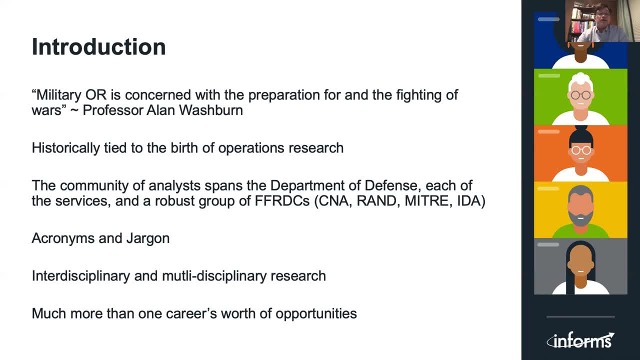 that they are incorporating the military and the Air Force and they're incorporating the operations research techniques as well, But each of the services has operations research that is embedded as a part of their, of their military force structure, And there is also a robust group of federally funded research and 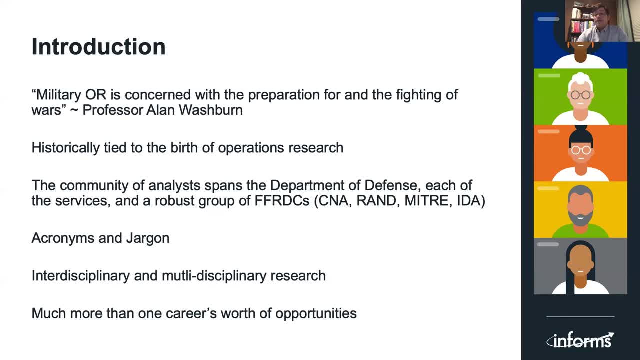 development corporations, and these companies have really sprung up as nonprofit organizations to assist the Department of Defense in solving some of these really demanding problems, And the Center for Naval Analysis, or CNA, RAND, MITRE, IDA Institute for Defense Analysis, are all examples of these FFRDCs that are run on. 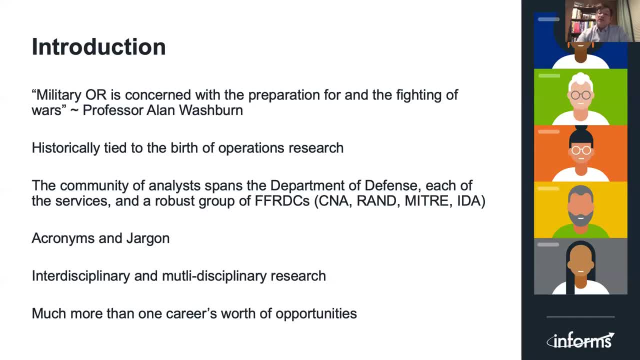 behalf of the Department of Defense. So one of the things you'll find in military OR is acronyms and jargon, and anybody that deals with this community just even for a short time has to take a step back and and really look and see what all these different acronyms are And as these kind 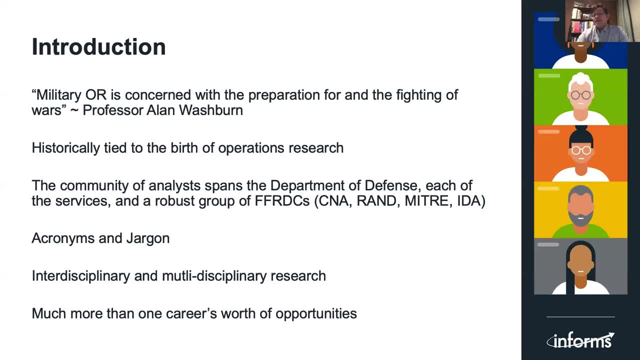 of acronyms come up. I really encourage the the young analysts to ask questions. I remember being in a meeting in Baghdad and I had met a British officer on a British, an American-Australian forecasting exchange and so I was a friendly face We. 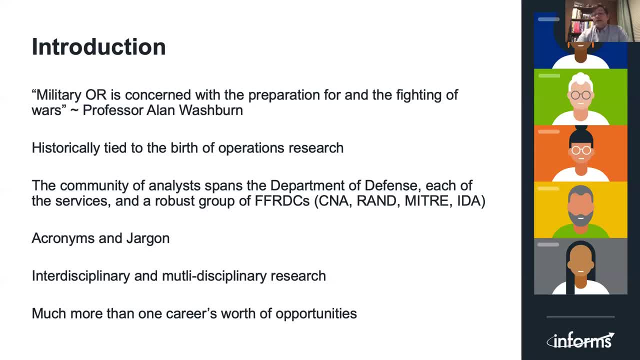 we got done with a meeting and he asked: was that in English? Because the amount of acronyms that we use as a part of our military speak can be completely overwhelming. But everybody has time to answer what the acronyms are about. So never be afraid to ask any questions on acronyms and 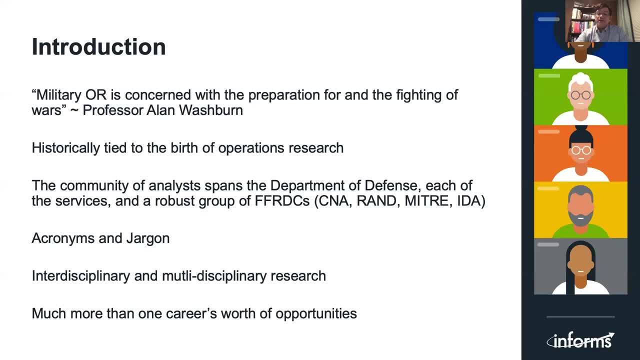 our jargon, And learning that and being able to speak is part of what you have to figure out when you work in this community Operations. research is definitely an interdisciplinary field And we work on multidisciplinary research problems as a matter of course, And when I take a look at 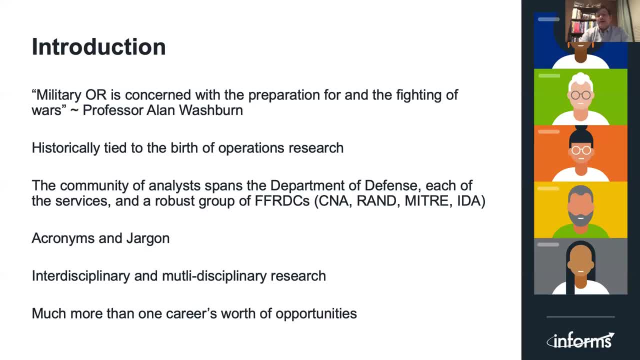 the things that I've been able to do over my career in military operations research I can think of in the Army. there's many organizations I never got a chance to serve in. I served mostly on the Army staff, the joint staff, the military academy And between that, my work in education. 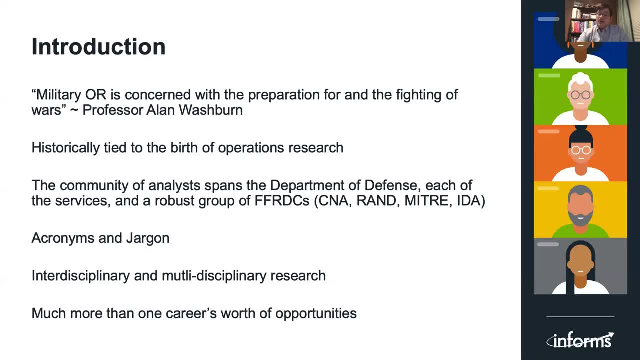 and my work on the staff in the Pentagon that filled up almost 20 years worth of operations research time when you throw in the deployments that we go on, And so when you think of the other things that people could have done, we have quite a bit of other work that is available. 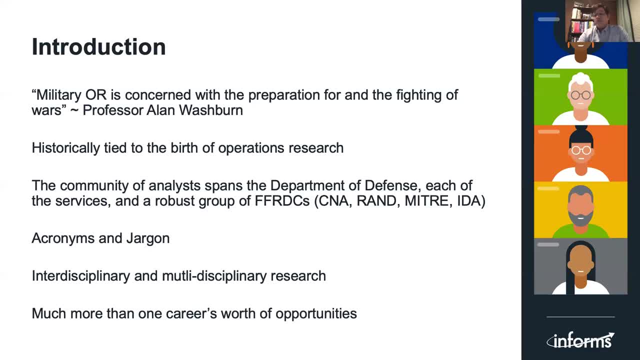 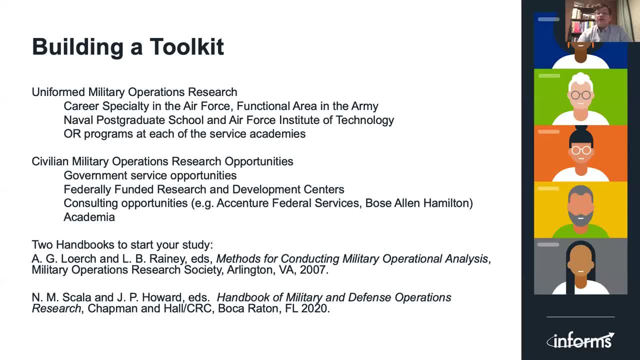 Force. some of their young lieutenants coming out of the Air Force Academy or coming out of ROTC will work as operations research analysts- their entire career- career In the Army. we have a functional area and officers come over as Army captains. 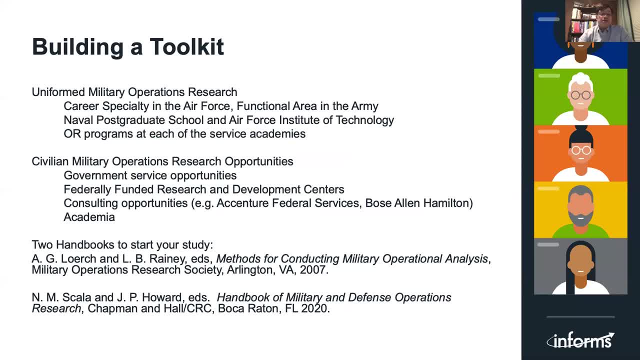 and the Marines and the Navy send quite a few officers to the Naval Postgraduate School to learn about the skills of OR and then bring those ideas back to the fleet and to the rest of their of their work. And the Air Force continues to send people to the Air Force Institute of Technology. 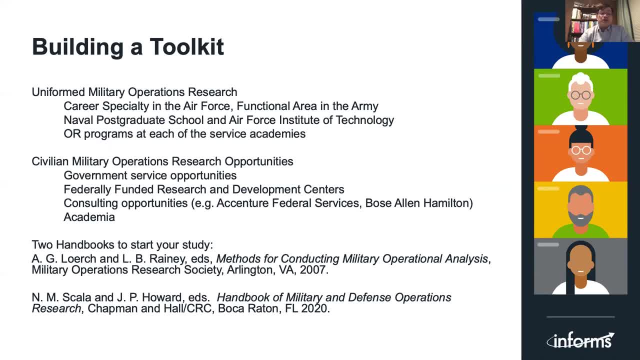 and those two schools, the Naval Postgraduate School and the Air Force Institute of Technology, train and educate a large number of our operations research professionals that serve in the Department of Defense And, in addition, we have operations research programs at each of the service academies where we teach our cadets and midshipmen about the fundamentals of operations. 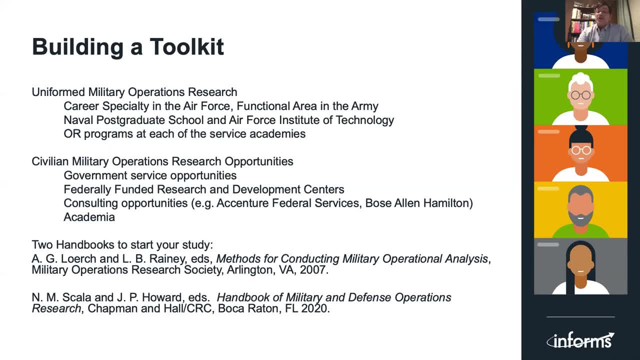 research. The necessary combination of math, science and engineering, appreciation for political science and history- the things that really make a great operations research analyst are things that all of the cadets and midshipmen will learn. So even those that choose not to major in operations research are well-posed to eventually. 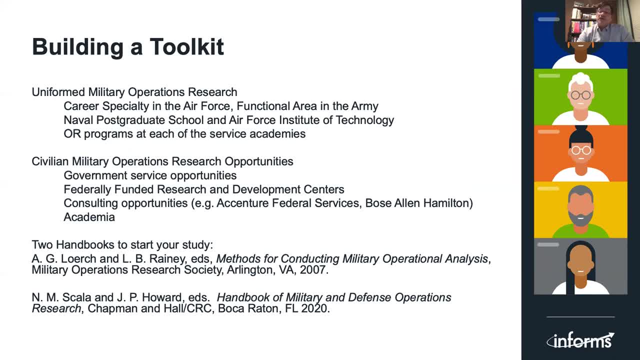 join the group of people that do operations, research for the Army. Now, likewise, there is a huge number of students and there is a huge number of faculty, and there is a huge number of faculty that are in the military and there is a huge number of faculty that are in the military, And so 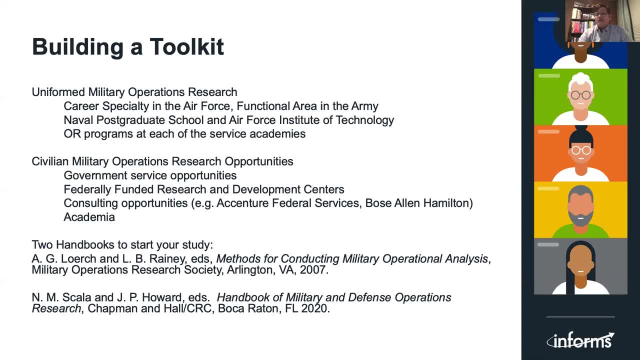 there are a lot of opportunities for them to get a degree in military operations research, And so there are a lot of civilian opportunities for working in military operations research as a civilian. There is government service opportunities. I was speaking about some of the organizations like the TRACC centers, the Center for Army Analysis or Test and Evaluation, a large 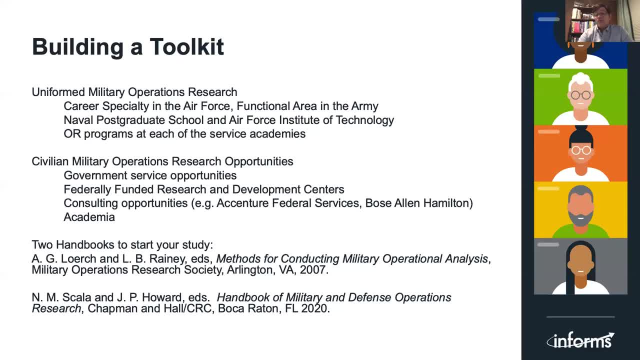 number of centers where they are nearly all civilian. They will be working with the military, But these private corporations are another opportunity to serve and to work on these kinds of interesting problems. And then there is a lot of the big consulting firms work, and there is 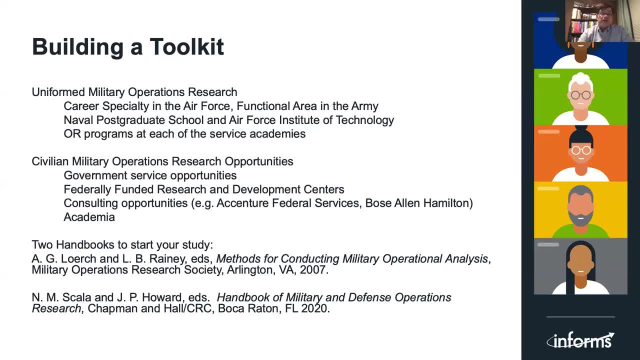 consulting opportunities where you can join a company, something like Accenture, Federal Services or Booz Allen Hamilton, and get a chance to work on on these problems. And of course, then there is also the root of academia And so the entry point for both- for a uniformed analyst as well as for a civilian analyst- to work. 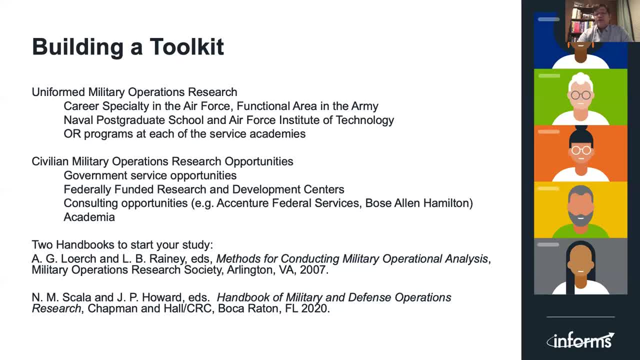 alongside them is going to be the technical background that allows you to enter into operations research as a field, And so if you are prepared to do operations research in any of the areas where you could perform military operations research or operations research, then you are going to be able to apply. 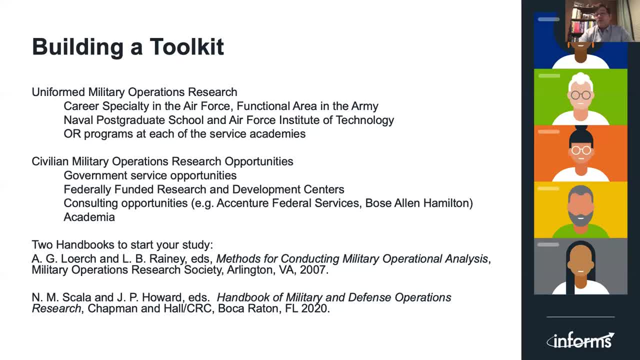 it to the military. It is just a different application. So, whether or not you are doing marketing, and we have operations research analysts working in marketing for the Army, as well as every company across this country, And so you end up with these same sort of problems. 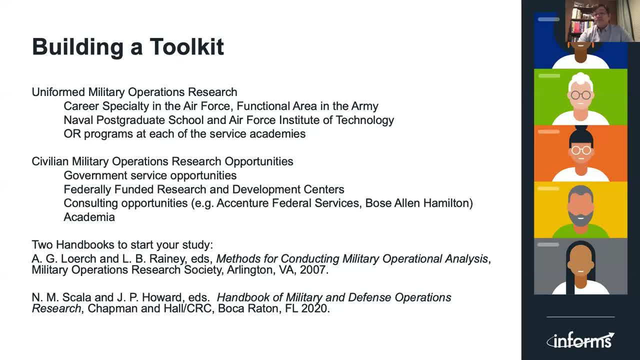 that are prevalent in any large company that the services have to work on as well. So there really is a lot of opportunities for you to join and to work on these kinds of problems. There are two handbooks that I would like to highlight for you, as you kind of think about. 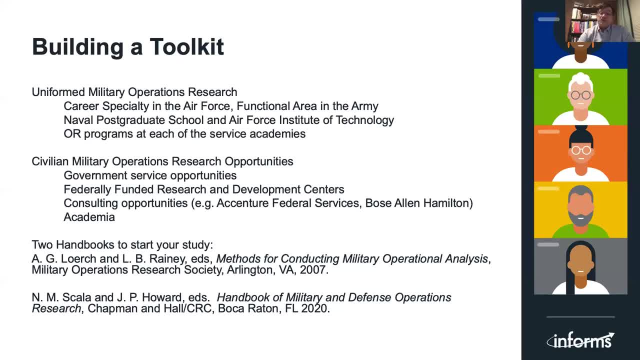 the beginning of how you would do operations research tailored to the military services or to military and security problems, And one is the methods for conducting military operations analysis Which Andy Lurch and LB Rainey put together for the Military Operations Research Society. 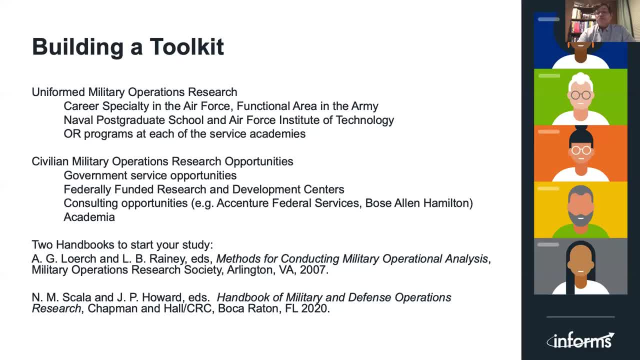 And it really highlighted an attempt to share some of the wisdom that had been learned. that is often only on PowerPoint slides, Because a lot of what we do influencing decision-makers in the Army ends up on PowerPoint slides and doesn't actually get written down and shared in journals. And so what Lorch and Rainey were 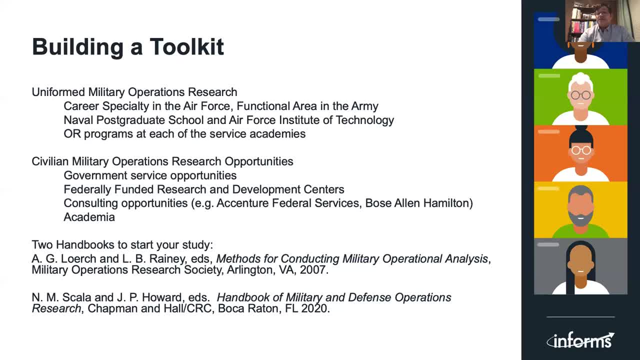 really trying to do was to find a way to capture some of those lessons and to bring them out into methods of conducting military operations analysis. And then Natalie Scala and JP Howard have a handbook on military and defense operations research, which just came out this year, which 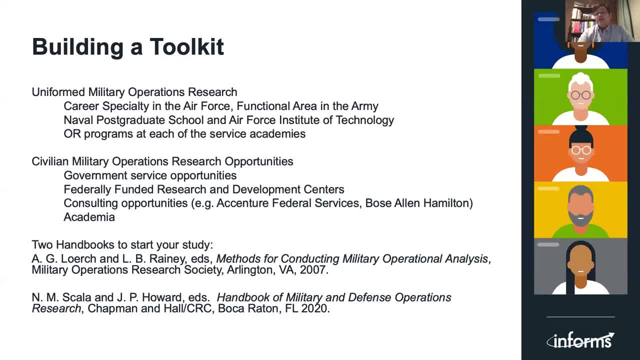 details a lot of different ways to do military OR and has some examples, And so I offer those both as two places to begin your exploration of military OR if you're interested, And if you're either interested in doing it in uniform or interested as a civilian and applying some of 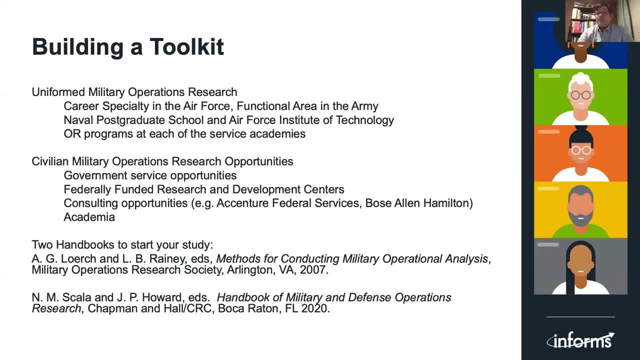 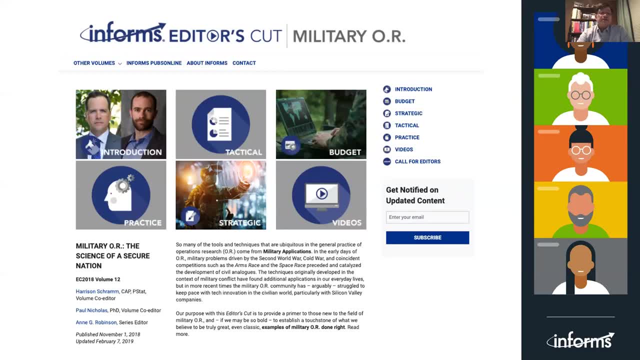 your tools to these kinds of problems. these are two great handbooks to take a look at, And one other great place to start is to take a look at the editor's cut, And we really have a great opportunity to take a look at the problems and some of the good research And 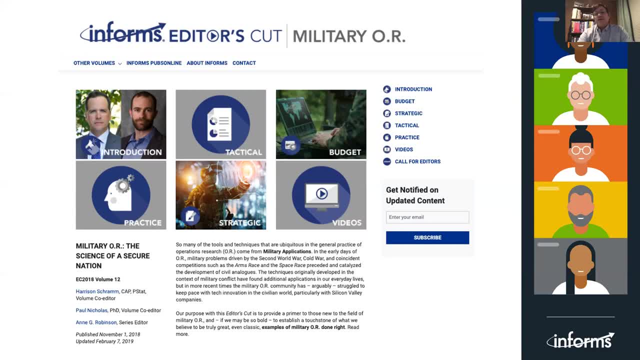 Harrison Schramm and Paul Nicholas put together this editor's cut looking at the areas of budget, strategic operations, tactical and then practice, And it really is an opportunity to look at some of the work that's been done across our community and is also something that's 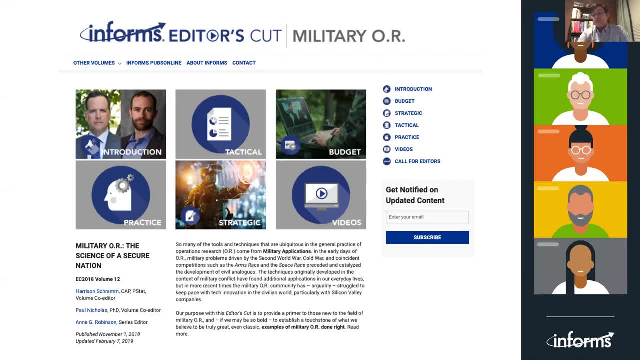 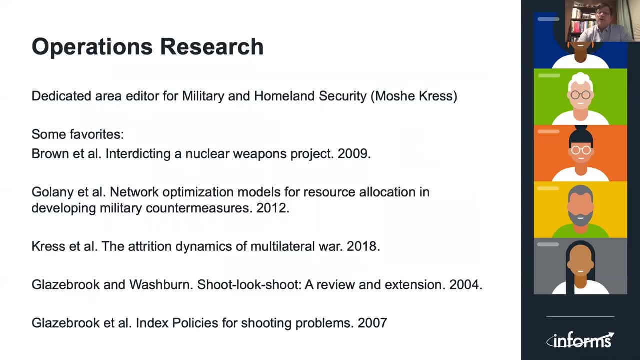 available to all of us on the INFORMS website as a part of our membership. So if you take a look at the areas where the vast majority of our- the papers that are written- end up operations research- is definitely one of the places that houses a lot of the military research. if you're looking for military operations research, 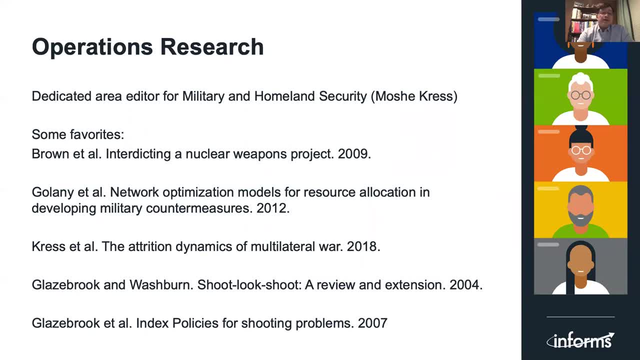 we have our own dedicated area editor for military and homeland security and Professor Kress is out at the Neal Postgraduate School and they're in my paper. I'll explain several of the papers that are in in operations research that are from a military standpoint, but in talking with the the area 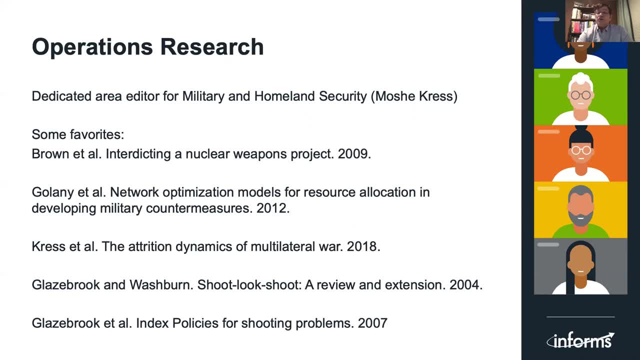 editor. there is papers that come in every year, and so it's a. it's a place where both you can submit your work as well as look for for new work coming out, and, although not highlighted in the paper, I'll explain several of the papers that are in the operations research. 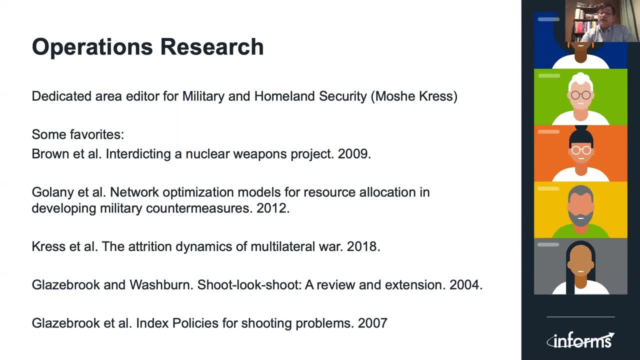 there's been quite a bit of recent work in intelligence, surveillance or reconnaissance, looking at the- the role of drones, and looking at some of the- the ways that you could do routing for drones- and so that there really are a lot of very interesting problems, some of the ones here that I 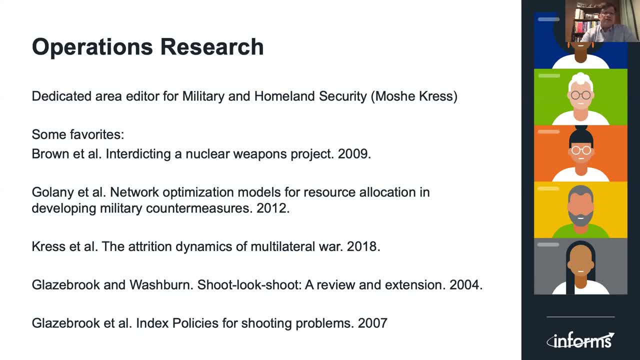 have highlighted Brown at all, looking at interdicting a nuclear weapons project, where you they had a really interesting paper that was looking at the way to to interdict- in this case Iran's nuclear weapons program. if you take a look at Galani, at all the 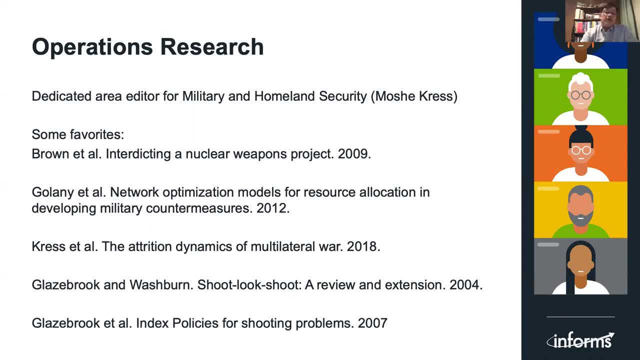 network optimization models for resource allocation in developing military countermeasures is another fun paper, and you start to see some of these words that you're very familiar with. if you are interested in network optimization, then this is a great kind of paper to read and to get started, where you can see how your favorite 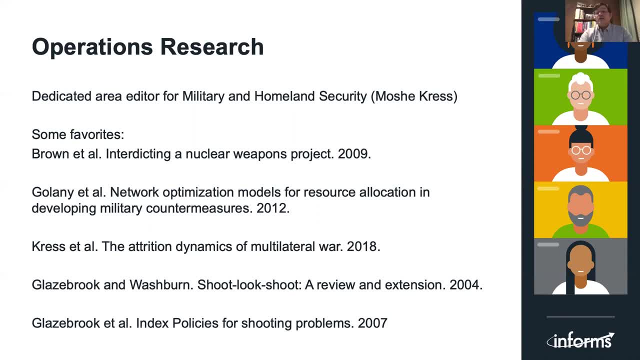 tools can be applied to some new application areas and crest at all after the attrition dynamics of multilateral war is is a neat paper that extends the, the Lanchester equations, and then glaze book and washburns, shoot, loop, look, shoot. a revision, review and extension, and then 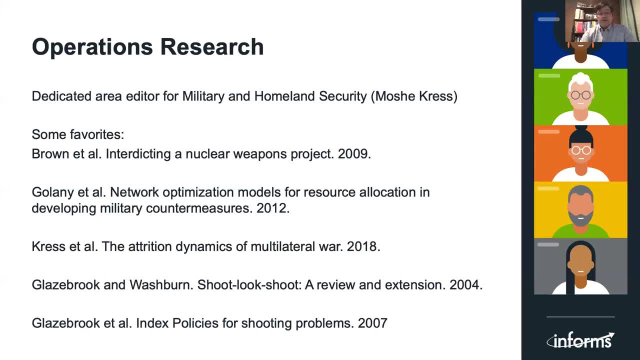 glass. look at all's index policy for shooting problems. help to show how sometimes these classic problems can really came out of military or and and how you can you look at expanding some of these problems and with this is one of those areas where they were looking at air defense and getting a. 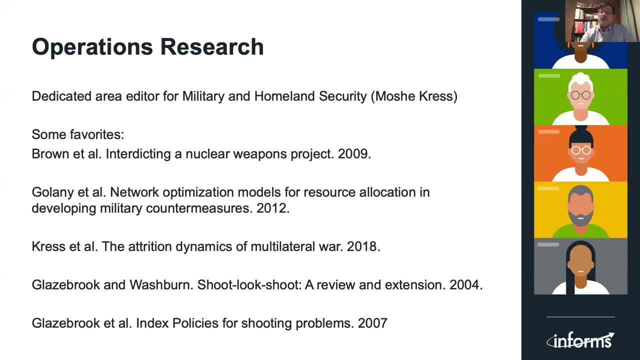 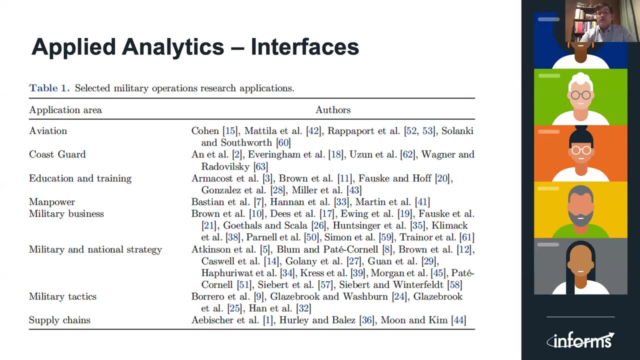 chance to look at how air defense would work with regard to some of these, these shoot, look, shoot type problems. so next, the another popular place to look for work on military or is in applied analytics or the journal that used to be known as interface, and so I've highlighted several areas. 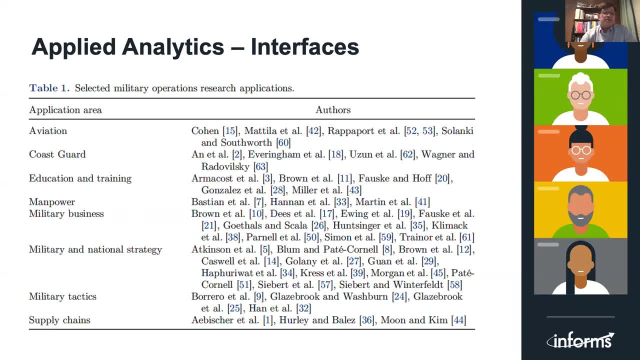 here where you can take a look at different kinds of applications and some some papers that you can take a look at their kind of app, some classic examples. so I've got some applications here that are in the aviation sector. with the aviation they've a lot of interesting work, everything from from crews and trying to figure. 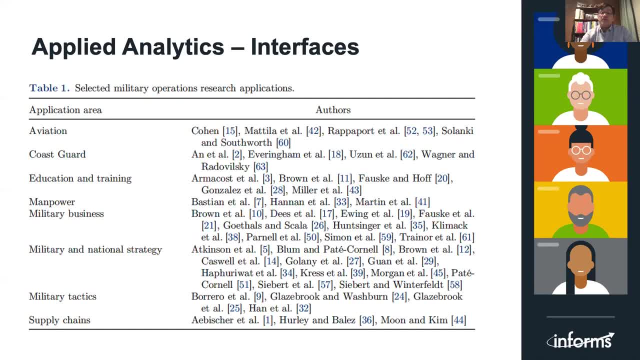 out how to do crew rest, to routing some really another really fruit, really a very nice area to do work in. the another area is the Coast Guard. the Coast Guard has quite a few applications where you look at how you defend an area, the, the roles of ships in that kind of defense, the interdiction of 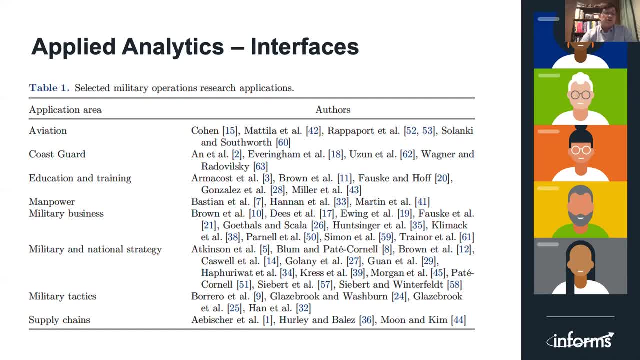 drugs at sea. there's some, some nice applications in the Coast Guard, and then another area that we have that gets quite a bit of writing about is the education and training, and so we look at how education and training will be done in the military or- and there's some papers here that talk about- 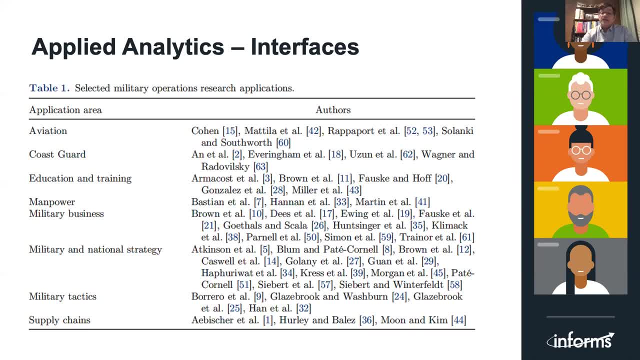 the, the training of OR analysts at the academies and at the our graduate institutions. another popular application area is manpower and really military business type problems, where you take a look at everything from power or the different critical infrastructure and how you could relate these things to how you work on bases and camps, posts and stations and really look at how you can. 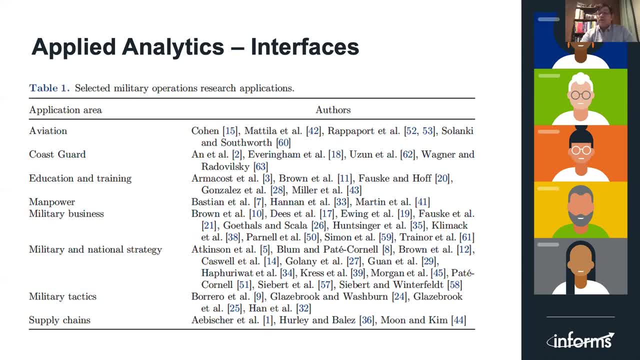 really solve some of these problems that are important across the critical infrastructure structure, but really these things that really look at applying the the rules of business into the running of the military as opposed to the fighting of the military. there is some nice papers on military and national strategy where you look at a lot of game theoretic constructs. 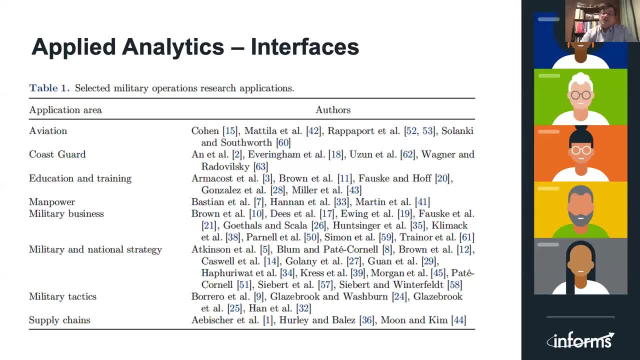 but how you can apply these OR tools to the different levels of war, be it tactics, operational or strategic level of wars, and really looking at military and national strategy. and so then that brings it to the military tactics. there's the, the group of papers that look at the more tactical level of war, which is another area. 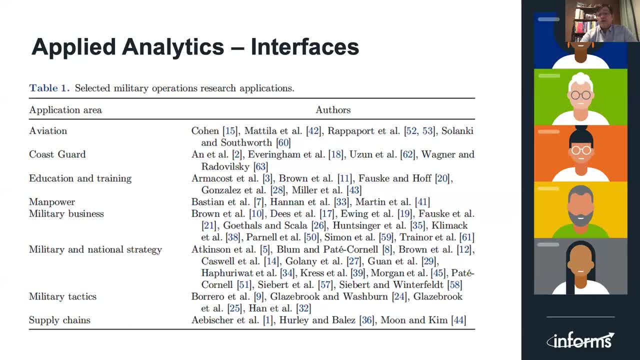 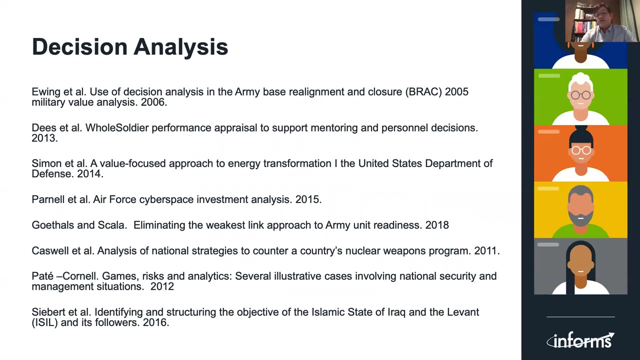 and then supply chains and there's some, some really interesting papers over time that have talked about everything from a multi-echelon logistics to just in time and the. the work in really is a very interesting set of research for our community. Then the last group that I'm going to discuss are: there's quite a few papers that come out. 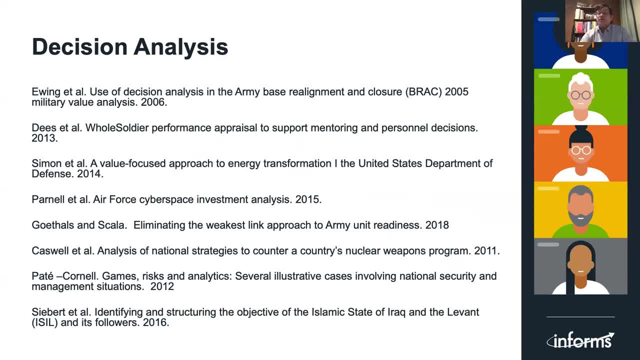 of decision analysis, And I think this makes a lot of sense because so much of what we're doing is trying to provide decision tools or decision support to commanders and other staffs, And so we get some examples here of some great work that was in the Informs Journal: decision analysis. 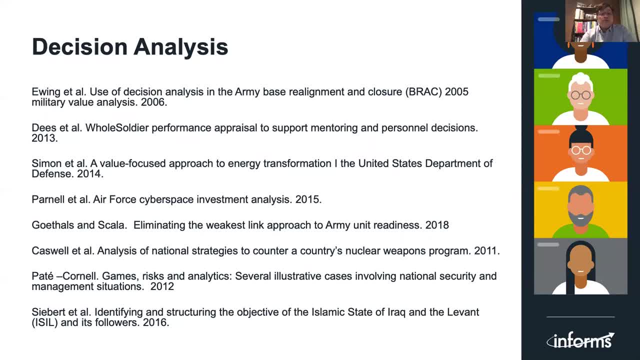 So Ewing et al did a piece on BRAC where they were looking at how to make the best choices to shut down some of our posts that we decided that we're thinking we didn't need anymore. Dees et al did this whole soldier performance appraisal system where they were looking at 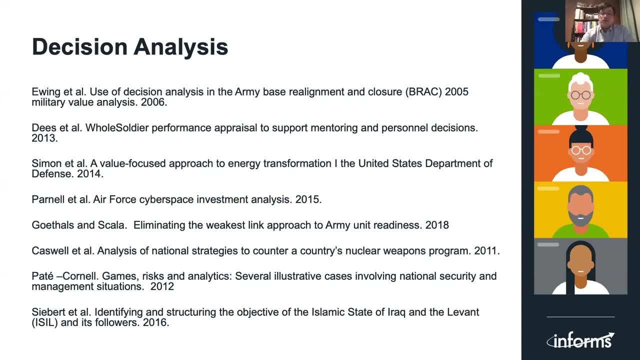 different ways of counseling junior soldiers and then doing an assessment process of the entire soldier to try to find ways to do better mentoring, Whereas we hadn't really done any counseling or reports started at the NCO level. So really taking a look at how you could do those kinds of evaluations at the soldier level, 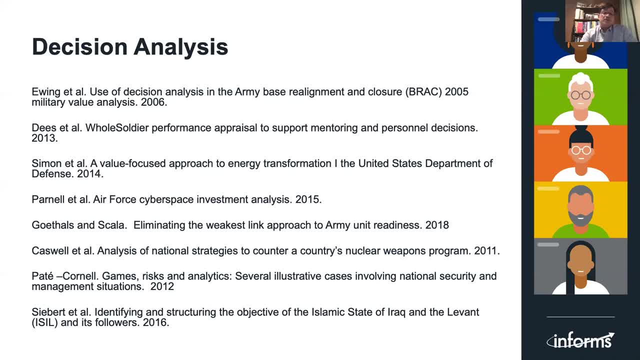 Simon et al looked at a value focused approach to energy transformation. So another one of those things where energy transformation is a very important part of the NCO process, And so we're also looking at how people with たんgeqongs specifically think about how. 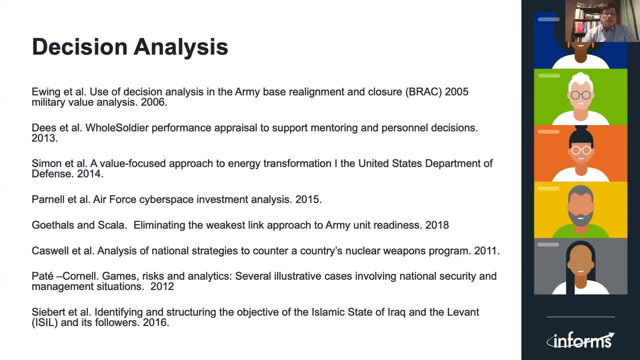 Transformation is something that Handy works across the board, And so so here was an example. we're looking at the in the Department of Defense Patane l at all. look at the air force cybersecurity investment and how they were doing their analysis, problems and scale. 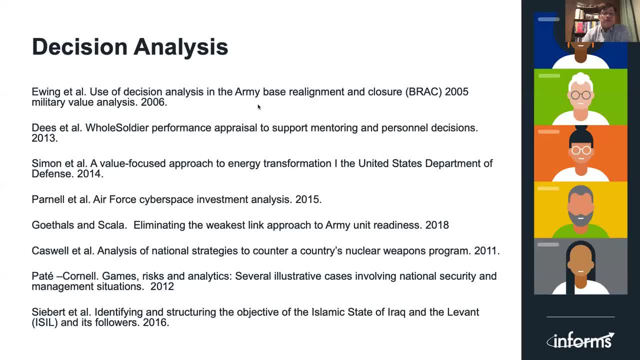 Goffles et al army unit readiness and trying to get away from a weakest link approach where you really just look at the worst part of readiness and it colors the entire readiness report. Caswell et al looked at national strategies for countering nuclear weapons, which was 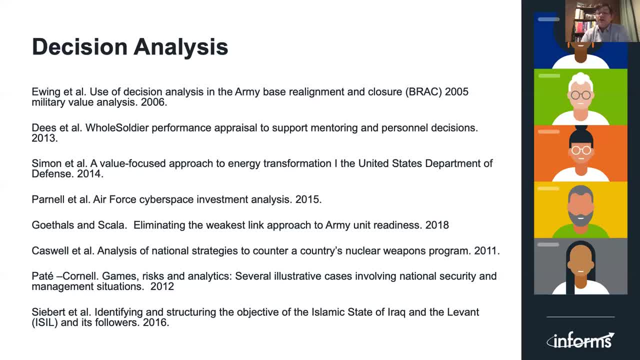 another one we saw earlier in military OR, but it's also had some nice pieces here in decision analysis. And then Pate Kornel has a nice piece on games, risks and analytics and looking at national security And that really there's a whole stream of research on this national security and management. 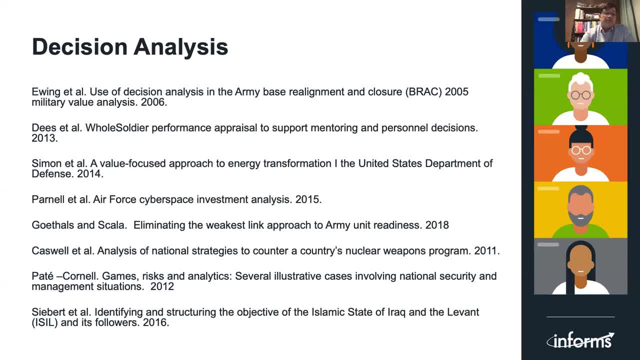 situations. And then Siebert et al have some nice papers looking at the objectives of the Islamic state of Iraq and the Levant, where you're really looking at how they were trying to structure the objectives and really work with their followers, And those are some really nice papers you can. 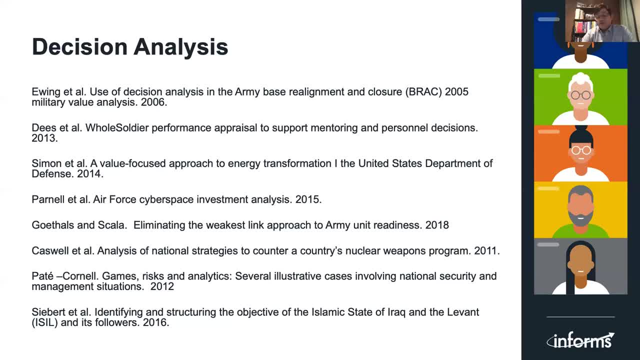 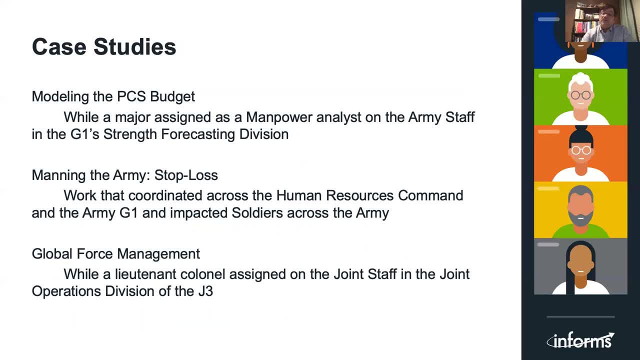 look at that. all are a part of the decision analysis. So for the second half of my talk, I'm going to turn to four case studies, And each of these case studies shows a different decision problem that I got a chance to solve. The first one was modeling the PCS budget And the PCS budget. 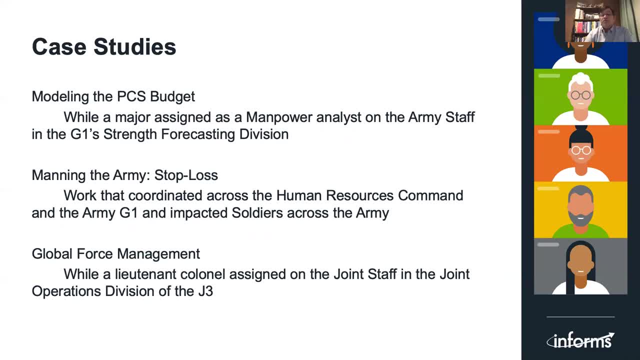 is the permanent change of station for soldiers as we are moving them from one post to another, And while I was a major and assigned to the Army staff, I got a chance to work on this problem as a part of the the Strength Forecasting Division. 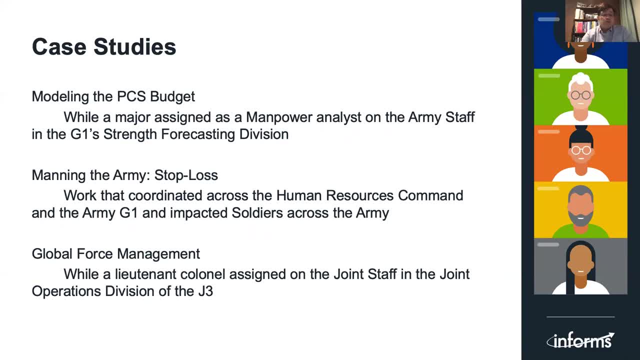 And this was supporting our budget, our budget work that we do every year. The second one is on Manning the Army and Stop Loss, And this was work that was coordinated across the Human Resources Command and the Army G1 and really impacted soldiers across the Army. 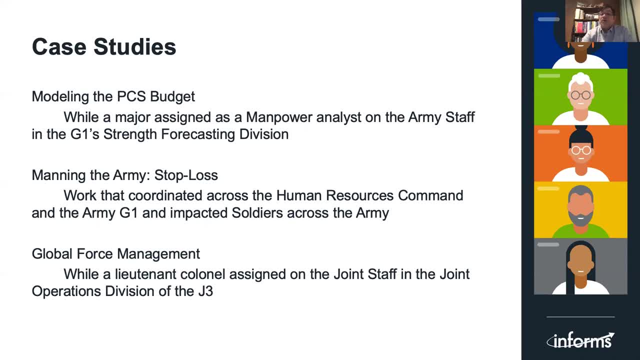 And this was work that I got to do with my wife, Colonel Mary Lou Hall, as well as Keith Olson, who was a long time member of the Army G1 and also worked down at the HRC and is currently working on the Army staff. 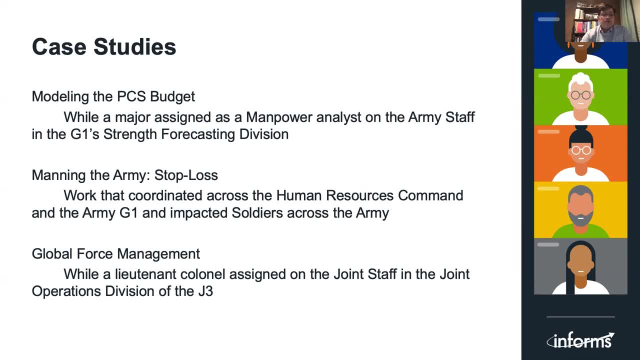 Then the last one that I'll talk about is Global Force Management, And this was while I was a Lieutenant Colonel assigned on the Joint Staff in the Joint Operations Division of the J3. I got a chance to work, and really worked hand in hand with- at the time it was Commander Keith Williams- 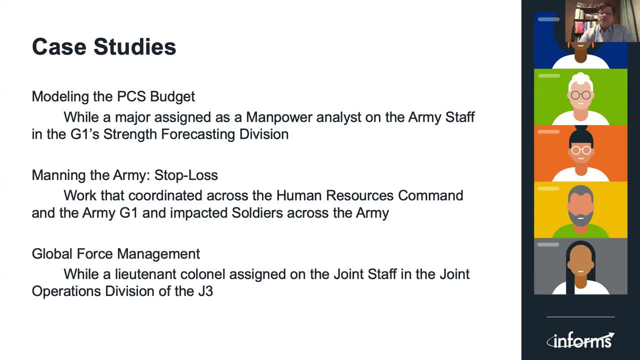 and he retired as a captain and was in the METOC field- the meteorology field, really in the weatherman group for the Navy, And we got a chance to work together on solving these issues of global force management and really trying to find a way, a strategic way. 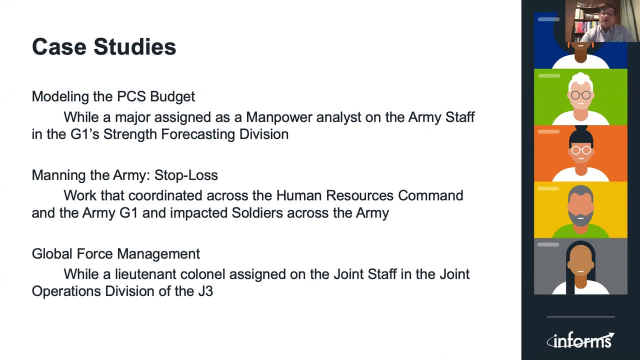 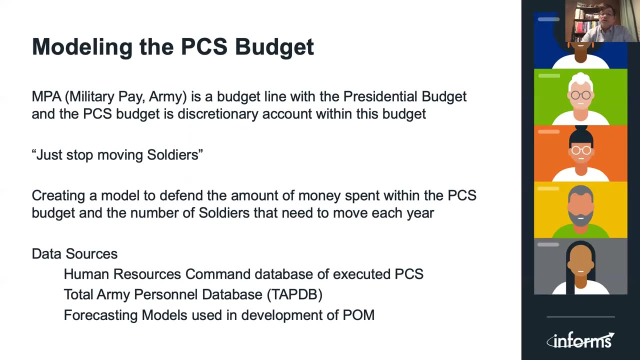 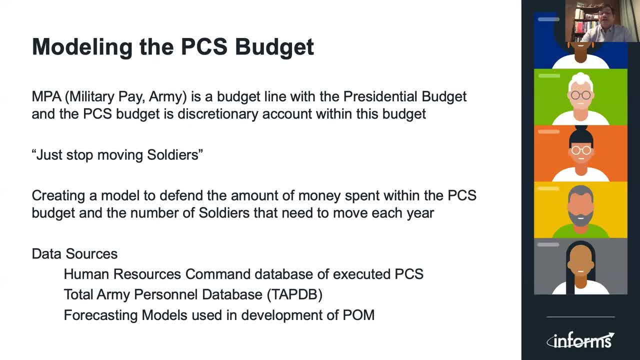 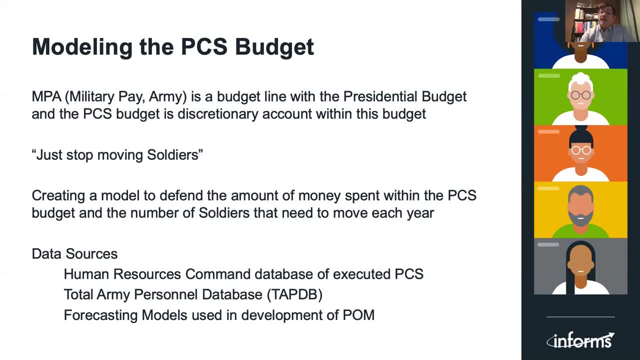 wow, that's something we can cut, that's discretionary And the idea kind of comes along. well, this is moving soldiers around. soldiers probably are happy where they are, or we could save money. just stop moving soldiers. And it really is one of those issues where 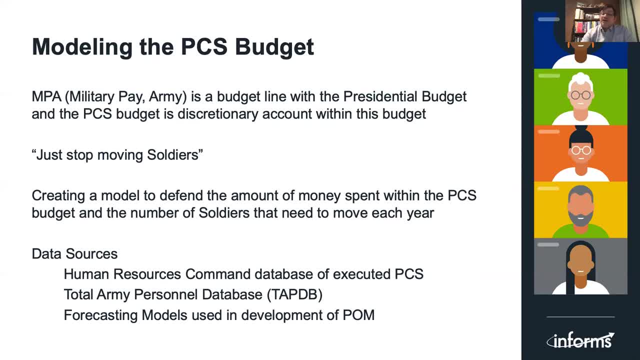 the discussion can be shown by a little bit of data analysis and some modeling, that the Army is always going to be moving soldiers, that the PCS budget is going to be pretty similar from year to year And we can get a chance to take a look at the different. 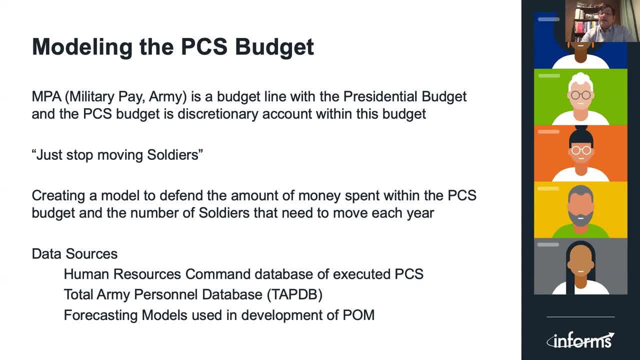 kinds of moves that we have every year and really identify how much flexibility there even exists within what someone would think of as a discretionary part of the account. So I'm going to we create a model to defend the amount of money that we spend on the PCS budget. 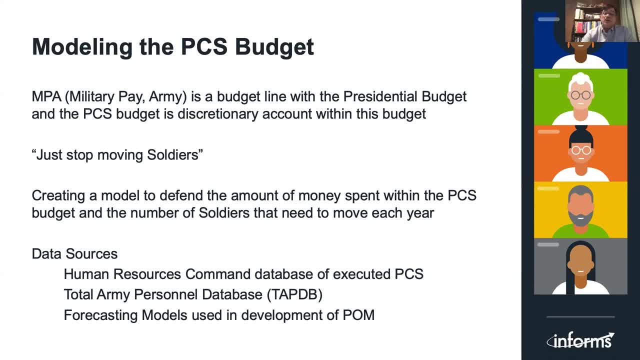 as well as the number of soldiers that need to move every year, And this is one of those problems where we had a really nice data source to work with, And so three of the data source that we use. one was the human resources command database. 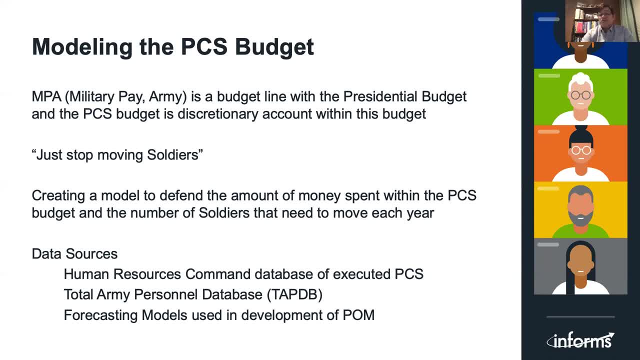 of executed permit changes, station moves, And so the human resource commander, HRC, kept keeps records of everyone that they ordered to move, And so it it that piece of data is able to be used also with the total Army personnel database, the tap DB. 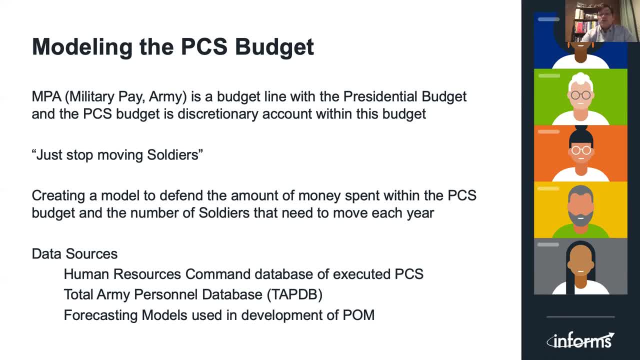 where we have all the information about the soldiers that are in the Army and where they're stationed, their ranks, our personnel data. And then the last piece of data that we used, or the last data source that we used, was forecasting models that we use for developing the palm. 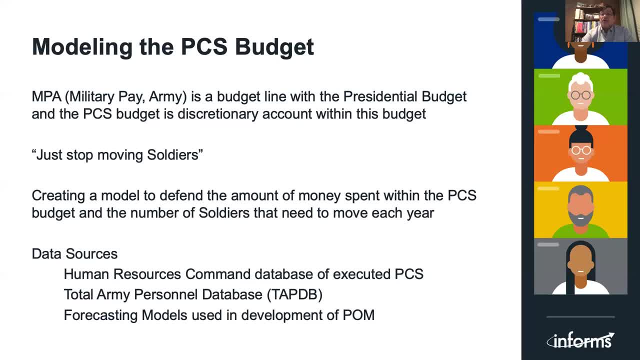 which is the program objective memorandum, which is our forecast that we produce in order to try to figure out what the budget will be, And so we forecast out and then look at the near years, for the budget and the out years is a part of the palm. 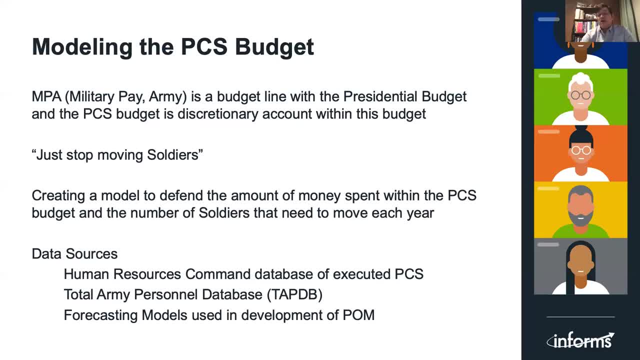 And so we've got within the Army G1, we have a forecasting models that we use to forecast the number of enlisted and officers that will be in each rank and grade, And so we use this kind of fidelity of forecasting to help with the forecasting of how many soldiers 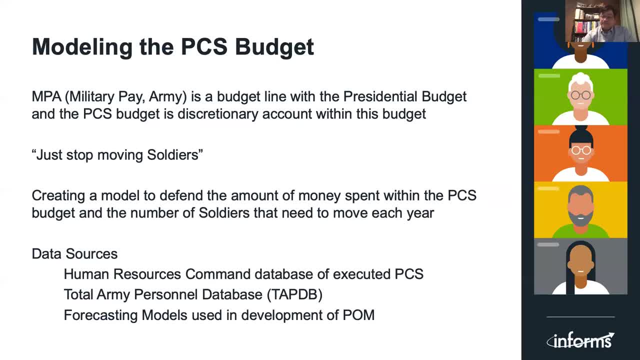 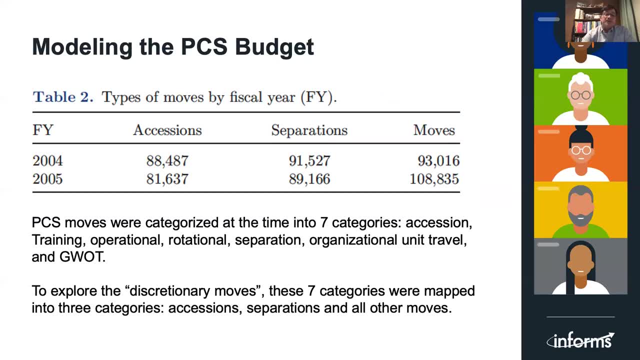 will need to move over the palm as well. So the first snapshot that we wanna take a look at is really looking at the type of moves by fiscal year, And so it's interesting that our moves were categories into seven different groups And there's seven categories. 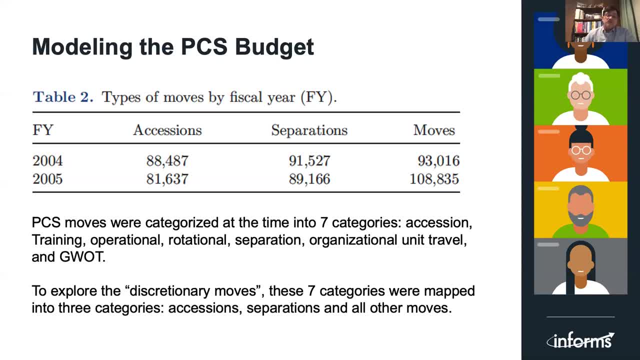 secession travel, operational moves, rotational separation, organizational unit travel and the global war on terror. So when you start thinking about seven areas by doing some data analysis, you realize that really there's a similarity where you can pull these seven categories down. 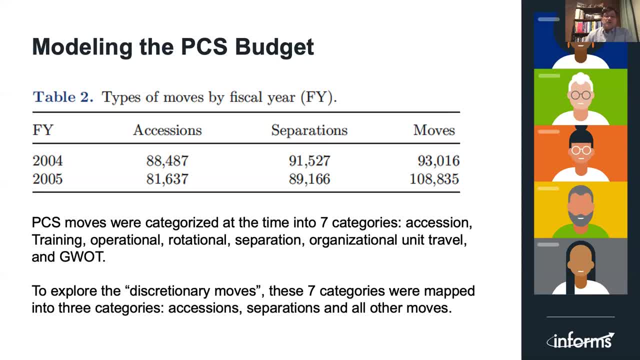 and reduce what you're looking at really into three categories, And so there is a secession moves, which are the moves that we have to do when someone joins the Army, So they go from becoming a civilian, from being a civilian to joining the Army. 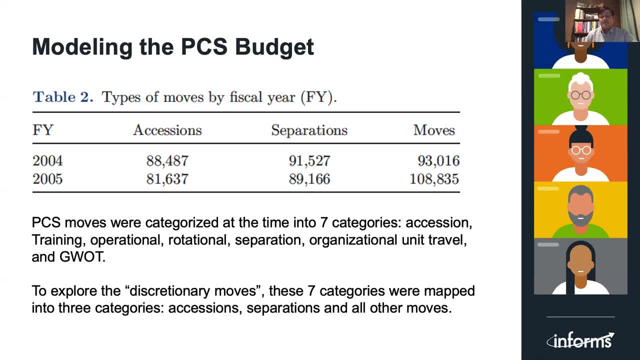 and we need to move them to their first duty station. So they'll need to go to basic training, they'll move to their advanced training and then they'll eventually get to their first duty station. But that secession move is captured and is essential. 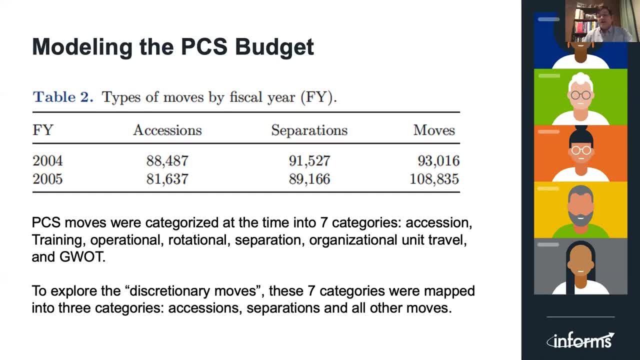 Another move that we have is separation, And so on the other side of the life cycle, when our soldiers separate from the Army, they are entitled to a final move, And so we move them wherever they would like to go within the United States or 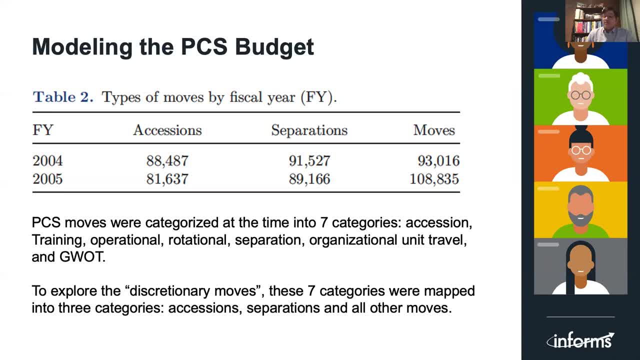 even overseas, depending on where they came on to active duty from, And so these kinds of separation moves is another large set And then so the last type of move is really all the other moves, And so all the other moves is everything else that we have to do across the Army. 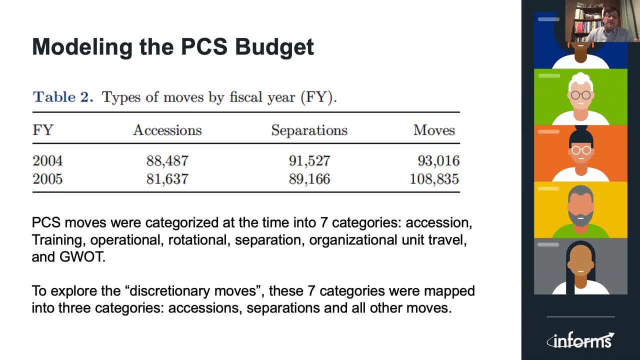 And so when you take a look at it in 2004,, we had just over 88,000 a session and about 91,000 separation moves, And you'll see that there's always going to be a relationship where, if the Army is shrinking, 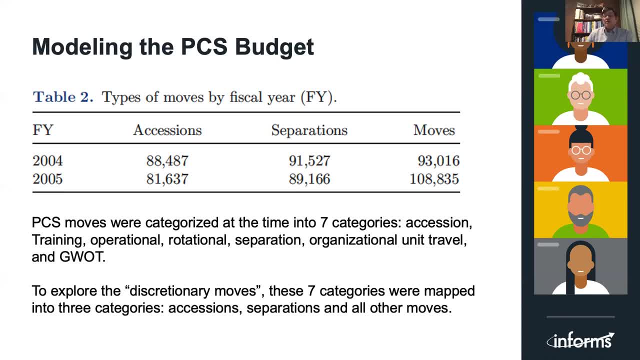 you're going to have more separation moves than you do a session moves. And if the Army is growing, you're gonna have more session moves than you do separation moves. And then you see that really about it's about a third. So a third are a session moves, a third separation moves. 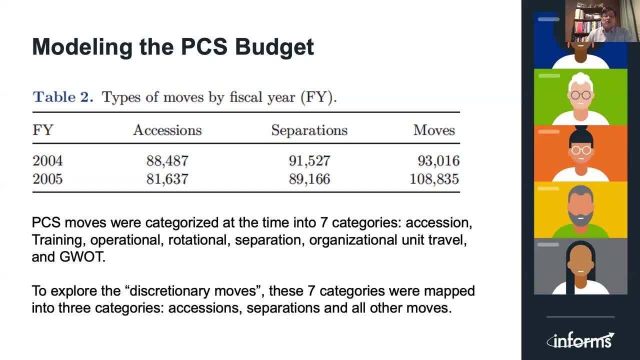 and then a third is all the rest, And so really two thirds of the moves that were accounted for across these two years were in the group. that really is not discretionary at all, but the ones that we have to do, And when you take a look at the moves, 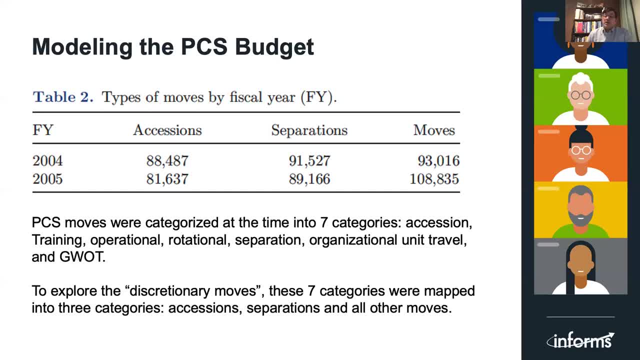 all the moves that you might consider discretionary. there's a lot of moves that we have to do for the readiness of the force, where you're moving soldiers to additional training over their life cycle or you're having them move to a new position, a new post, to get a new opportunity. 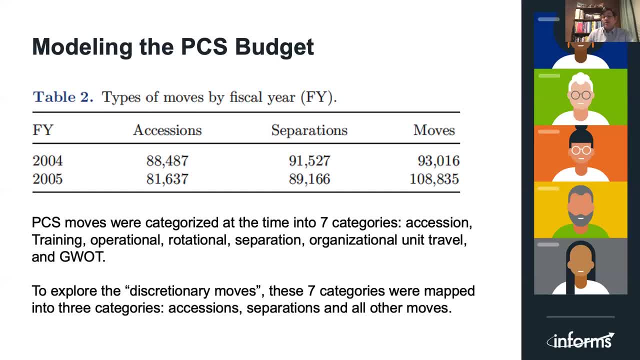 or when they get promoted. they are moving to a new post, to take a new job at a higher rank, And so these kinds of moves are also essential. but just as kind of a first blush on the problem, we can see where you can easily put a move. 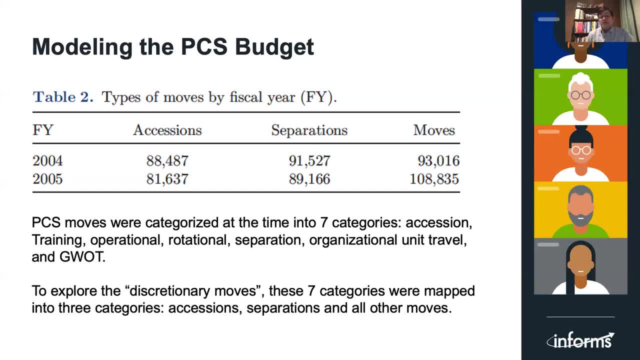 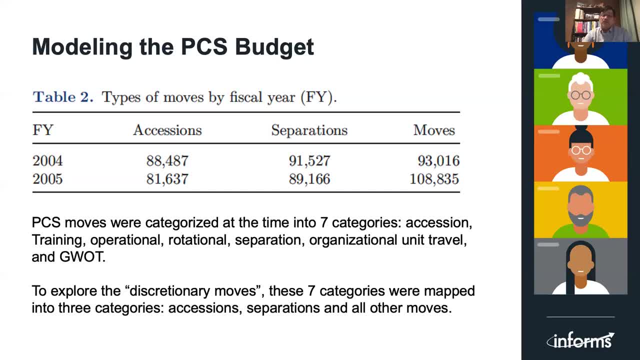 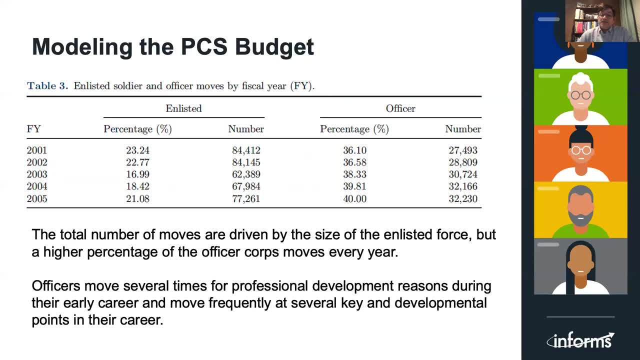 those leaving the Army, and then the moves that we do moving people around within the Army itself, And so the next interesting snapshot, and so the next interesting snapshot that we wanted to take a look at, is taking a look at the difference between enlisted and officers. 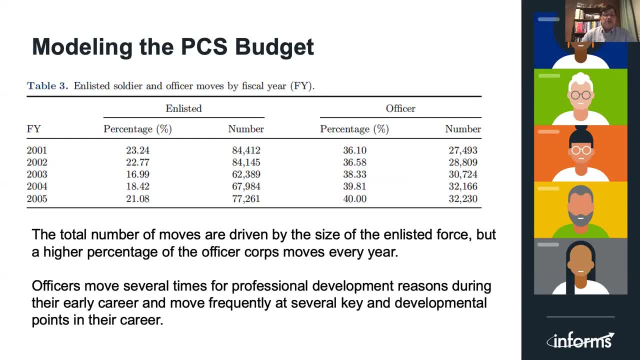 And so it's interesting, as you see over time, that the each year the percentage of officers that move is quite a bit higher than the enlisted moves, Whereas if you take a look in 2001,, we've got 84,000 moves. 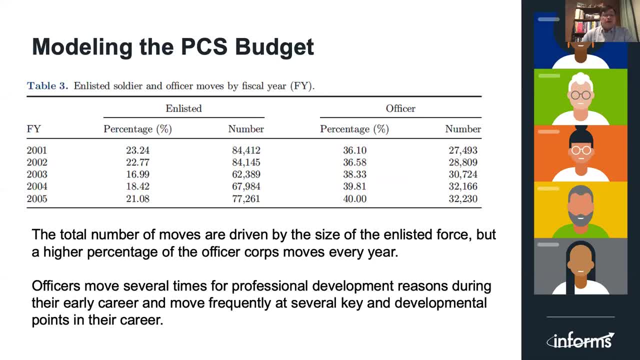 which accounts to about 23% of the force. And then for officers, we had 27,000 moves, which was 36% of the force. And so you take a look at this and you're saying, okay, why is the officer moves higher? Well, the officers actually have quite a bit of 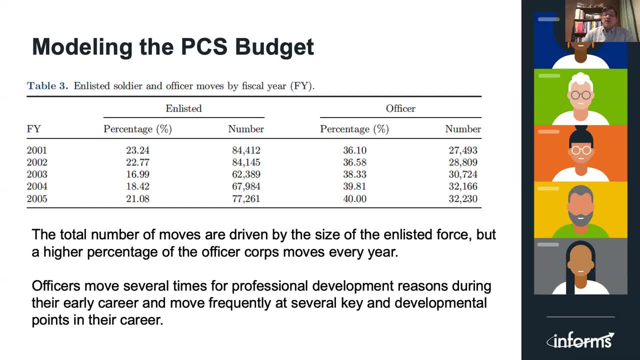 schooling that happens, And there's also several natural moves over the time- that somebody is a junior officer Whereas you work as a lieutenant and then when you get promoted to general officer, you're a junior officer, And so you have quite a bit of schooling that. 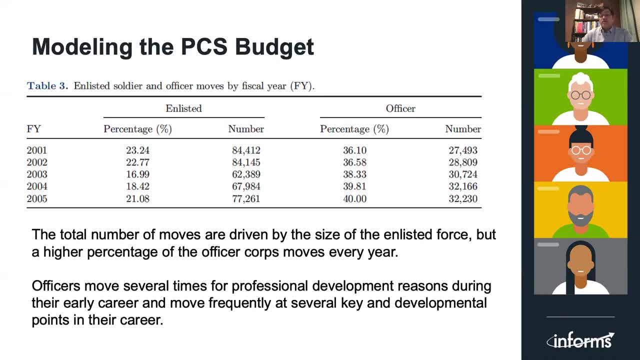 you have to PCS to go to school, And once you've gone to school for six months, then you PCS to the next duty station. So you end up with a couple moves within the course of a year. There's also some times in a career, like when someone is coming up on lieutenant colonel. 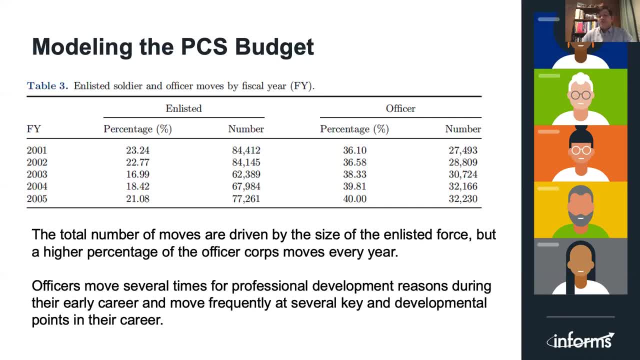 where they'll be PCS, to a place where they'll command, and then they PCS to go to war college and then they'll PCS somewhere to generally work, something like the army staff or higher level staff, And so you end up with a lot of these officers that get three. really it's like three moves in. 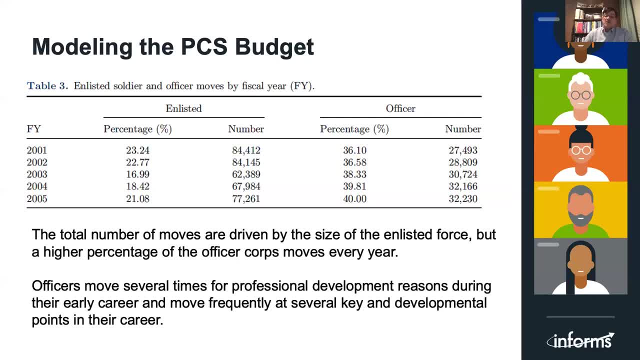 three years because of the way that the progression goes at that particular time in their career. But so we really take a look at here. you take a look at the differences and seeing the consistent percentage in officer moves and enlisted moves within the group. 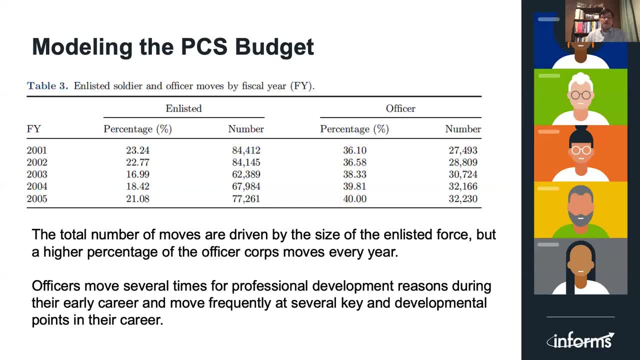 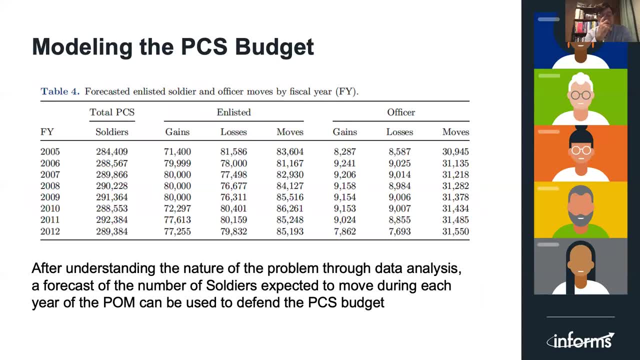 but there really is a difference between officer and enlisted moves, and so that will go into part of our modeling. and then next we take a look at the the actual, the PCS budget, and when we take a look at it we take a look at the gains, losses and and then the moves which we were talking about. 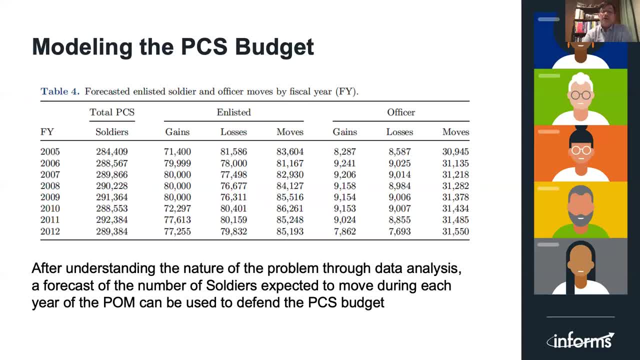 the moves is the ones that are more discretionary, but still the ones that are for the readiness of the Army, and you take a look at the, the total PCS moves for each year and you you see that there is some consistency. and this, this is something where, when we're sitting in 2005 and looking forward, we're going to. 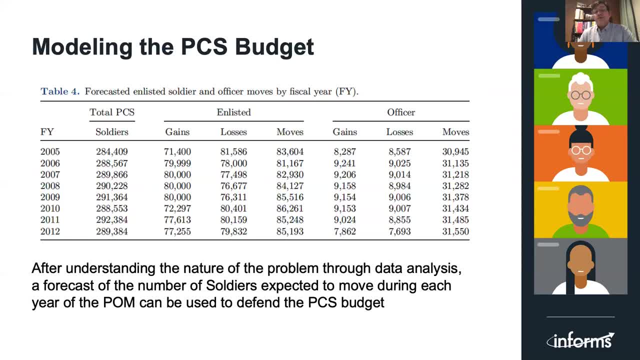 be looking at the number of soldiers that we believe will be in the Army each year. we have details on the number of promotions, we have the number that we expect to bring on to active duty, the ones that we expect to to come off of active duty, and so we're then able to to forecast, over this horizon, the number of. 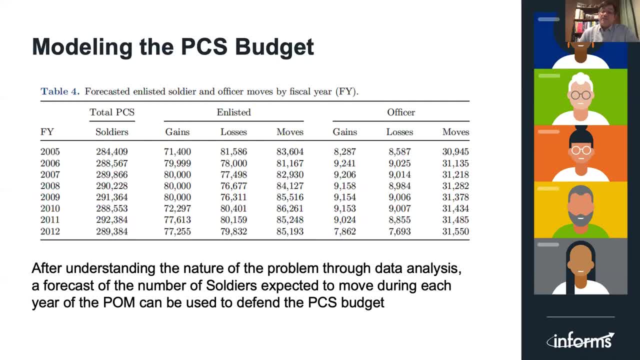 moves that we're expecting, and but by taking a look at at this kind of an answer, then you can start to take and price exactly how much these different moves are going to cost, And so when we took a look at this problem, it was really an example. 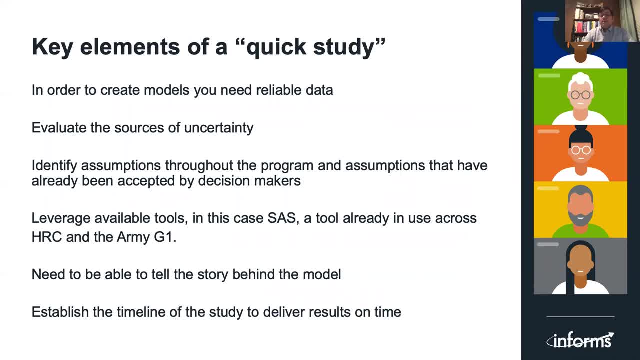 of the kind of elements of a quick study. The palm is something we do every year, And so when questions start coming about, why do we have a particular amount of money that we're putting against the PCS budget? it's going to be something that has a relatively short timeline and something 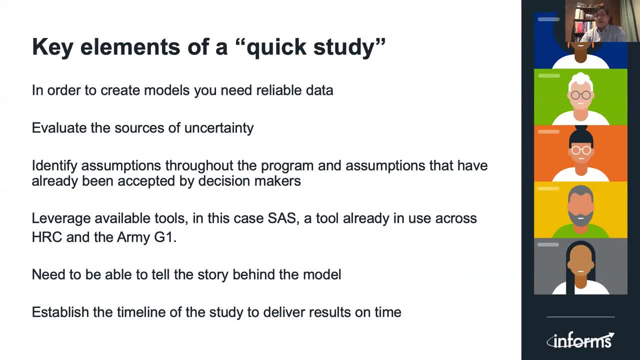 that they're going to want to have an answer on Now. often these kinds of questions, the direct leadership has a pretty good idea what the answer will be, but they want you to take a look at the data and really come up with the background and the hard examples and evidence so that they can 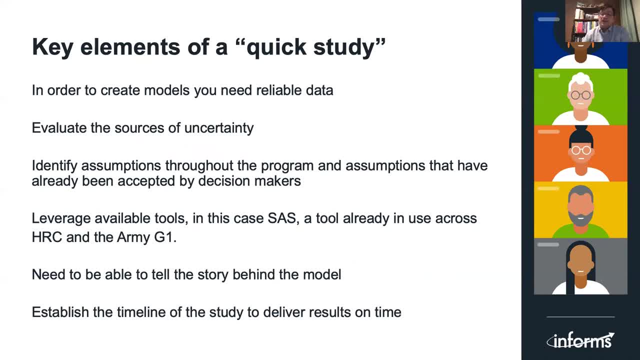 take this up And use it as exhibits on the hill, as we're defending our program, And so one of the things that you really have to do whenever you're doing these quick studies is where you're needed. if you're going to create a reliable model, you have to have reliable data, And there are quite a few. 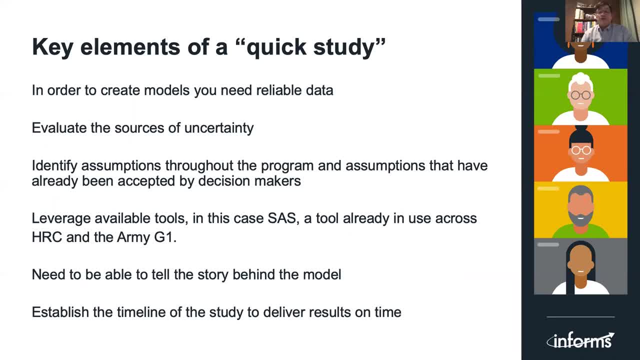 opportunities in the department or in the Pentagon, where we have quite a bit of data. And another thing that you really need to take a look at, you know, is evaluating the source of uncertainty. When you take a look and you're saying what? 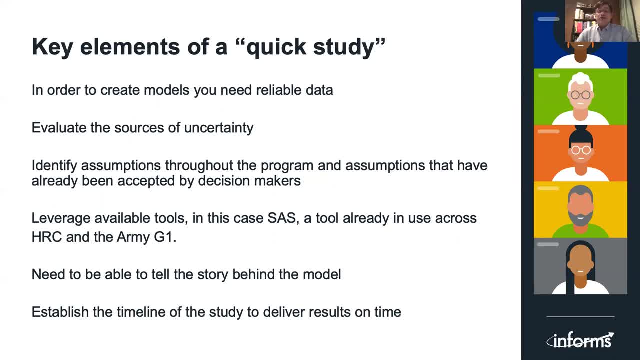 are the main drivers of the PCS budget, what are the things that are certain, what are the things that we've already decided upon? And this is one of those things where you get the chance to take a look at identifying assumptions and if the Department of the Army has made certain assumptions. 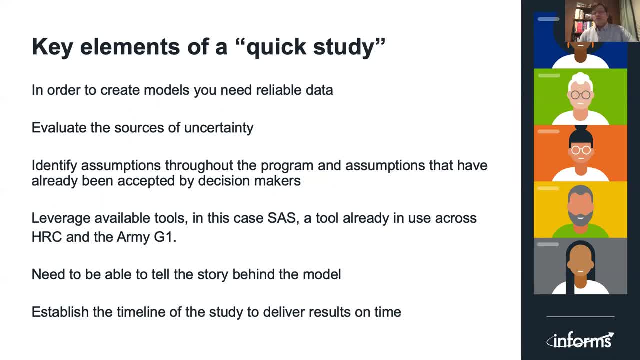 about what the size of the Army is going to be or other critical assumptions for the program program, then those assumptions have been debated and those have been accepted. The assumptions have been accepted by the decision makers, And so we have an opportunity to then. 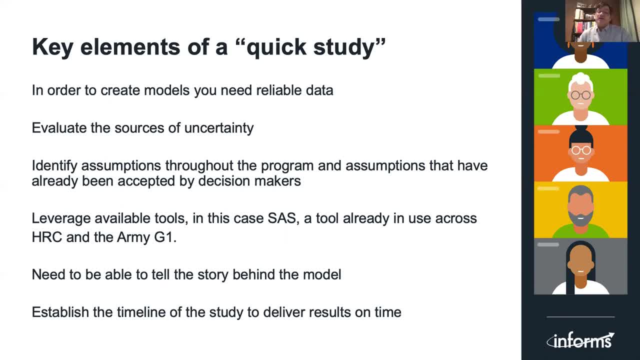 employ those assumptions throughout subsequent analysis like this. So another thing: when you're doing something quickly, you really have to leverage the available tools. In this case, we were using SAS, which is a tool that's already in use across HRC and the G1, but it also made it. 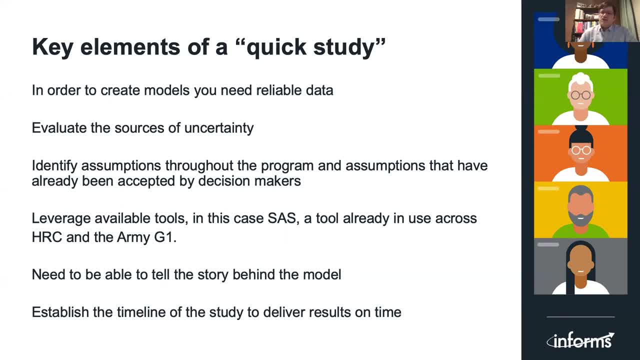 easier to use after we'd begun, as the major portions of this model would be creating the data snapshots based on the previous year's data, and then creating the forecast. It's also really important that you need to be able to come up with the story behind the model, And this is really 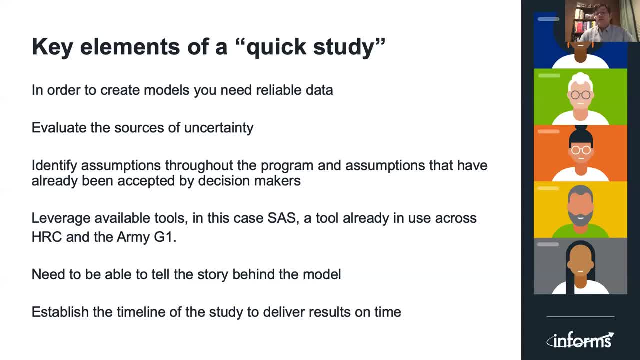 important, as the story behind the model is going to be, And so we're going to be able to come up with the story. So the story is going to go up through the leadership and explain why your model makes sense and is a good explanation of how much money it's going to cost for the particular item. 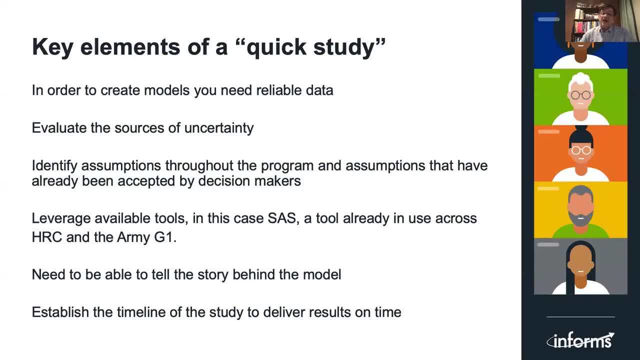 that you're researching. And one other thing is that the timeline of this study is crucial. There are some of these quick studies you'll need to do in a week and some of these quick studies that you might need to do in a month, Or it may be something that they want you to turn over. the 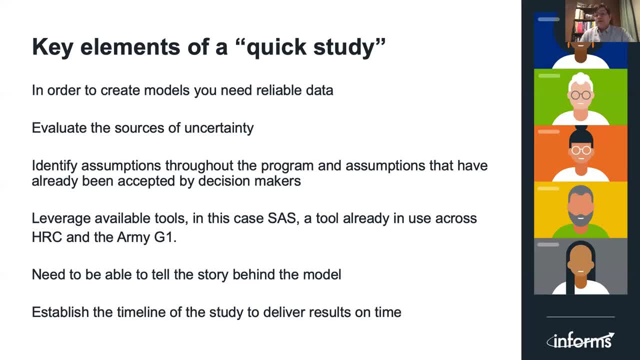 course of the day, It may be something that you realize you're going to be able to do every year, And so you then reflect upon getting this done and quite possibly, after it's due, you might revisit the problem to try to see how you could have a better model after it's turned in. 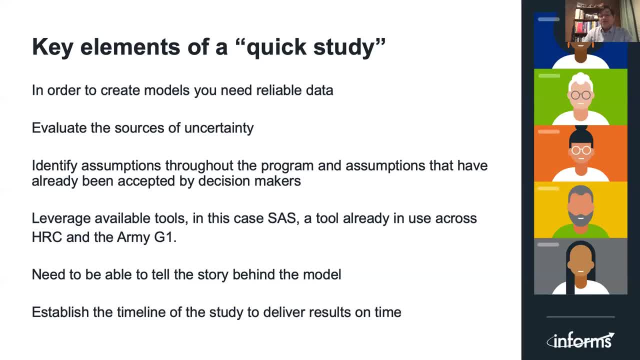 So just because it's turned in doesn't always mean that the analysis is done. A lot of times it makes sense to go back and review your work to see if you could have done it better, if there's different sensitivities and might be some different planning assumptions going forward. 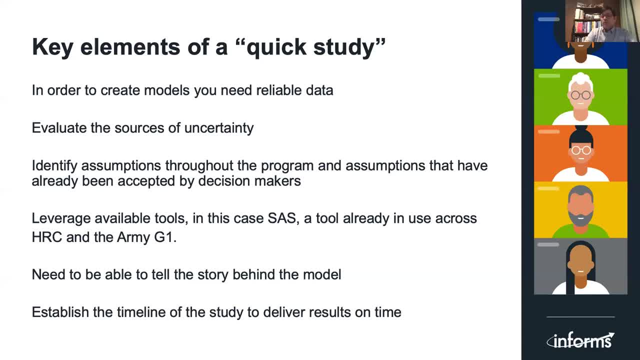 So that was an example of the type of work that I did when I was a major. and you end up getting assigned a particular piece of work by your division chief. the colonel And your branch chief lieutenant colonel, are going to give you a piece of work and they're generally going to be there to help you to come up with. 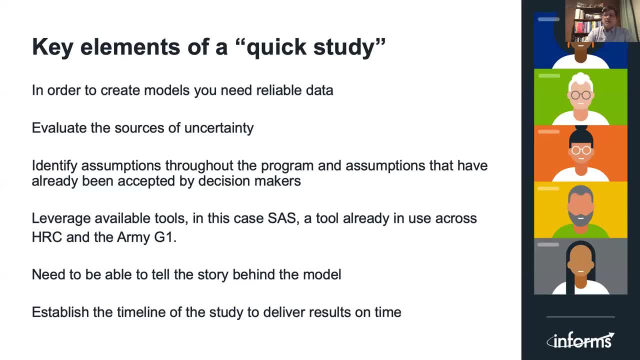 with these solutions and really it's a great kind of opportunity to do at the beginning of your time, when you're trying to figure out how to use the tools that you've learned in academia and to put these tools against problems, And one of the reasons why it really makes a lot of sense to have teams of ORS's working together. 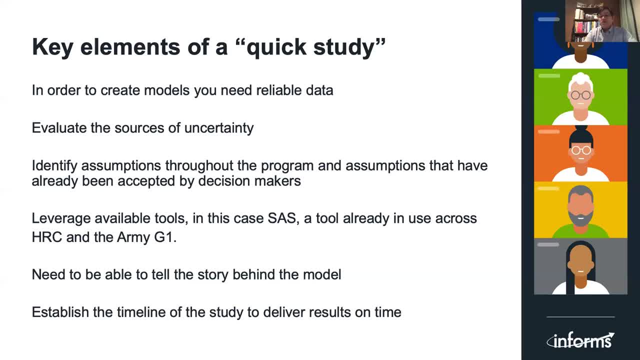 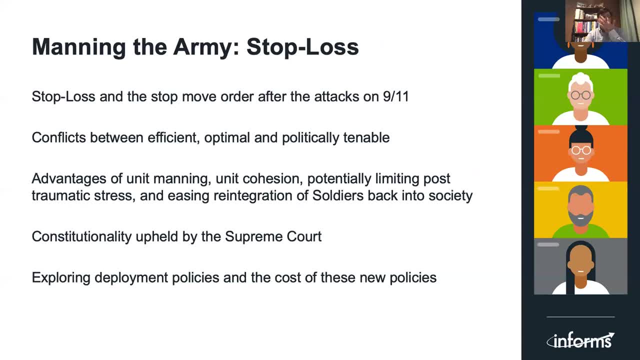 so that you You've got the senior leadership that is technical, as well as the officers that are working within the organization. So the next example that we're going to bring up is a example from Manning the Army with regard to stop loss, And so this particular 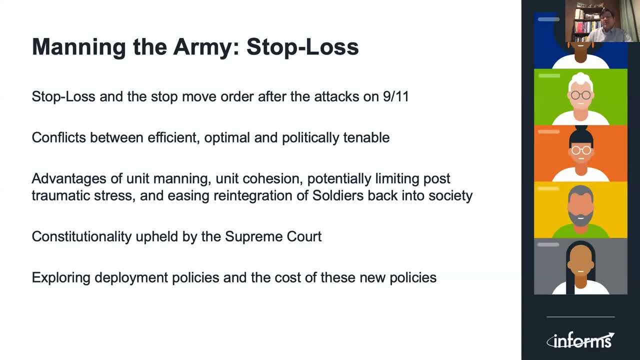 analysis had to do with the value of stop loss and the different kinds of deployment strategies that we could use to meet our deploying units, And so the stop loss and stop move order really came on after the attacks on 9-11, where, after 9-11, the initial response was just to have everybody hold what you got and figure out what we're doing, And then, as we went forward, 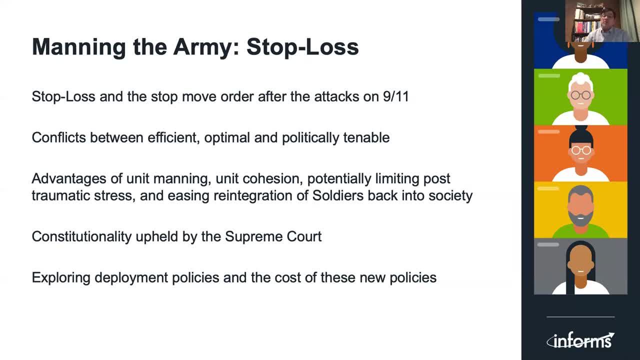 we wanted to keep everybody in Korea where they were. We were keeping the soldiers where they were in the United States and we wanted to prepare units for the deployments that would come up. So you start to get this conflict between the efficiency and what might become considered optimal distribution. 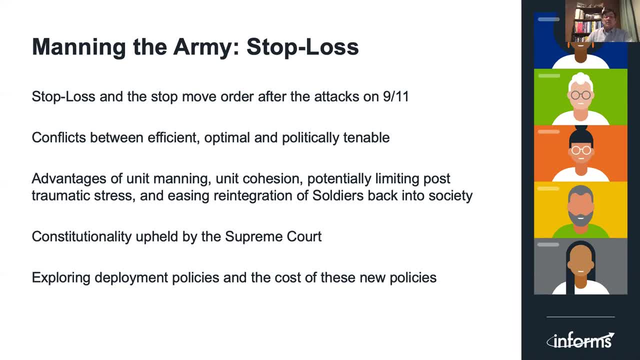 and really what is politically tenable. When we take a look at a concept like unit manning, which is really building a team, having a team, train, deploy, redeploy- all as an organization. it's something that was one of our lessons learned. 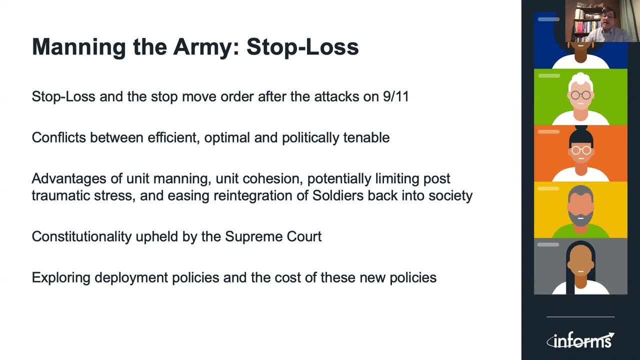 or one of the suggestions coming out of Vietnam was the value of unit cohesion and minimizing the individual replacements in theater, And there was some work believing that this would potentially limit post-traumatic stress and would definitely ease the integration of our soldiers as they come back into society. 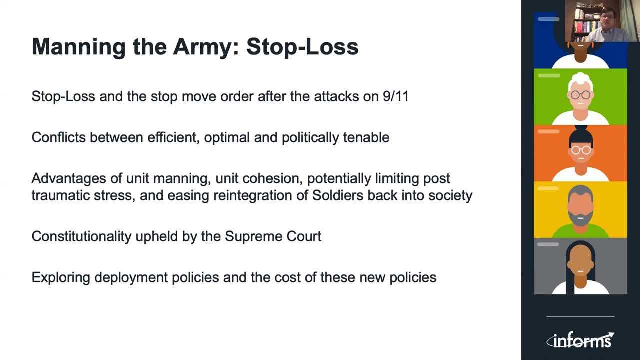 And so there was a lot of good reasons why stop loss and unit manning was something that we were gonna take a look at And, if you think about it, if you're gonna send a team for deployment, if you're going to leave them in theater together across 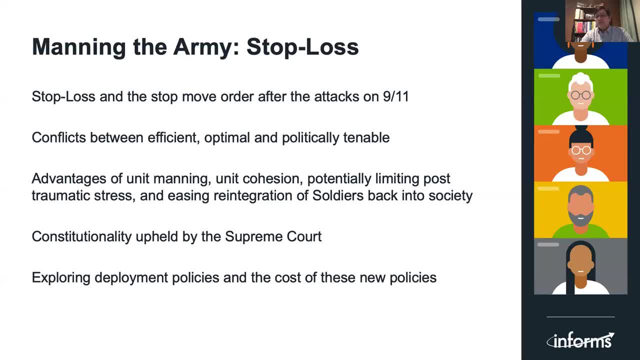 you're always gonna have some replacements that have to come into theater, as people need to be replaced, possibly because they were injured, possibly they had some important schooling they needed to do. There's going to be individual examples of why we would want to move people in and out of theater. 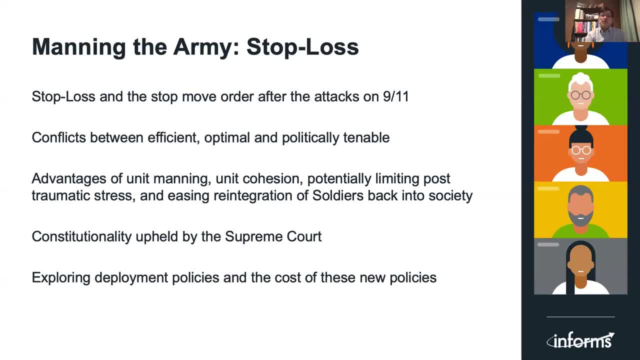 But by a general policy of everyone deploys together, everyone redeploys together. it minimizes this turbulence. Now, the contract that soldiers have signed for years has this extension built into it. Most soldiers are serving only a portion of their eight-year obligation. 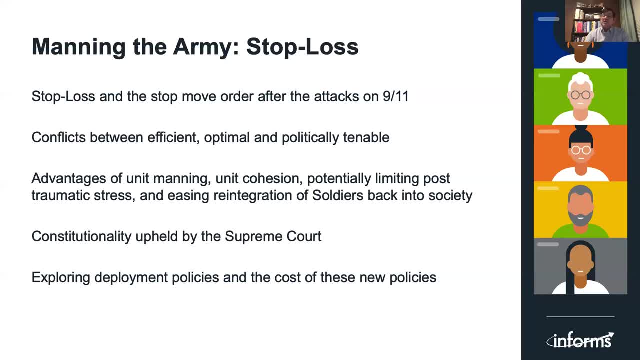 And so when somebody is finishing up their three-year obligation, they have an additional obligation that's in the reserve component. And so these kinds of contractual obligations, these kinds of contractual obligations, these kinds of contractual obligations, and what was actually signed by the soldiers? 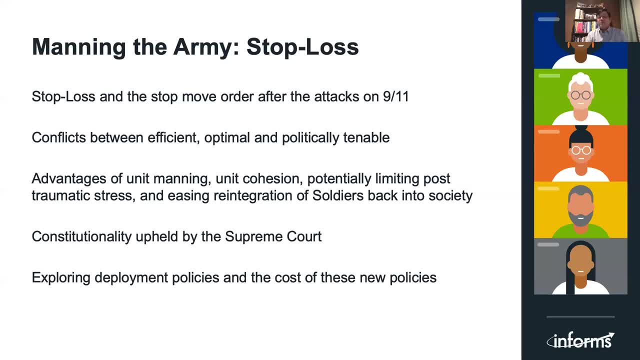 when they're coming into the Army was constitutionally upheld by the Supreme Court as being something within the authority of the Army and the Department of Defense to do. However, as existing policies started to be looked at and as we were looking at exploring a different deployment policies, 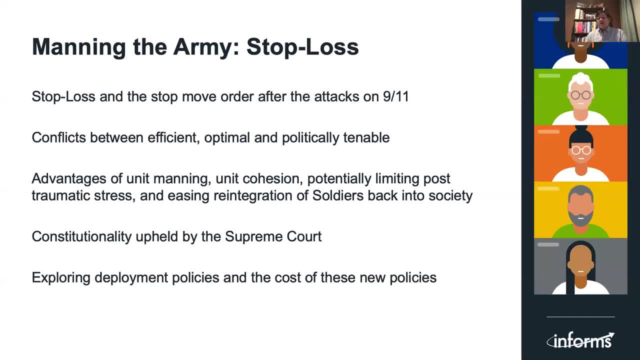 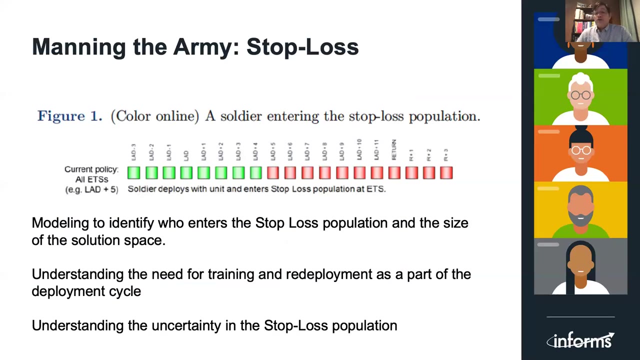 you really take a look at, well, how much does it cost if we didn't extend anybody's contracts, Or what are the different decision points that you can make as you take a look at this problem of stop loss And one of the things you find is that you don't even know. 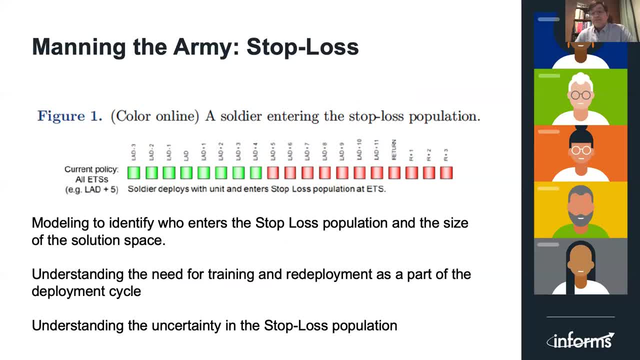 how many people are going to be in the stop loss population. So in this particular example, we've got this green bar across the bottom and you'll see that it says LAD minus three. LAD minus two. So these are the months going up to the arrival in theater. 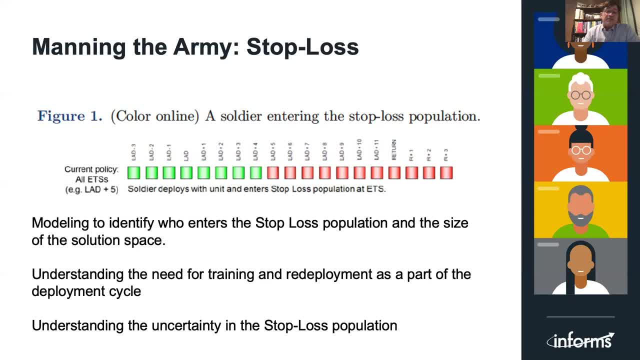 which is LAD, And this is an example of a soldier that would enter the stop loss population five months after they were deployed. Well, one of the things is that they don't have any obligation to re-enlist until they're at the end of their term. 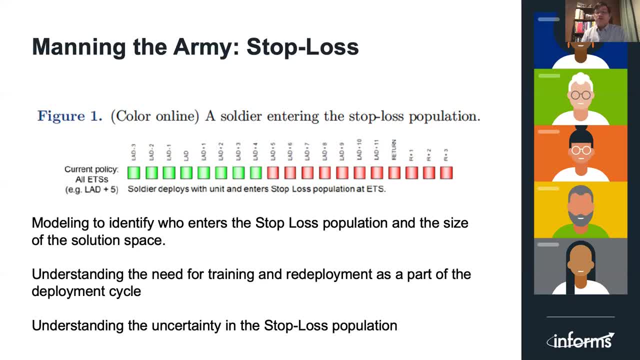 We found that there was a lot of times when re-enlistment bonuses and such that they would be required to re-enlist until the end of their term. We found that there was a lot of times when re-enlistment bonuses and such. 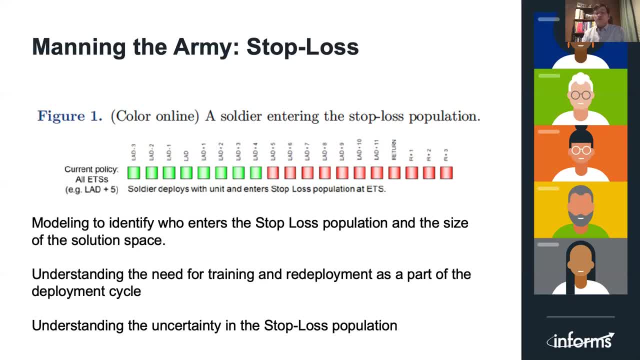 would fluctuate and there might not be the right bonus before they were deployed, but the bonuses in fear would be tax-free, And so there was a lot of interesting incentives for soldiers to not truly share what their intentions were, And there was also a lot of extensions where people would 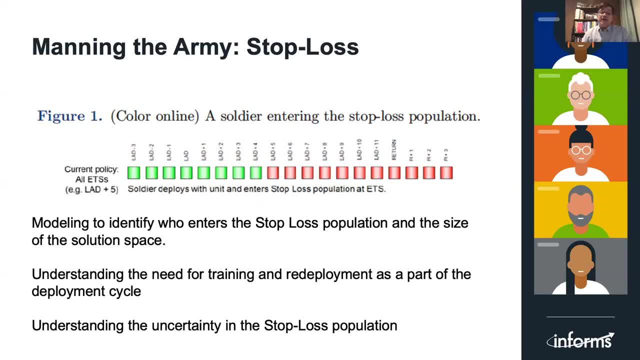 be given the opportunity to extend through the deployment, And so you're really taking a look at an unknown, because there's the soldier's action and they never actually become stop-lossed until they go past their contractual obligation. And so this soldier would spend the beginning of 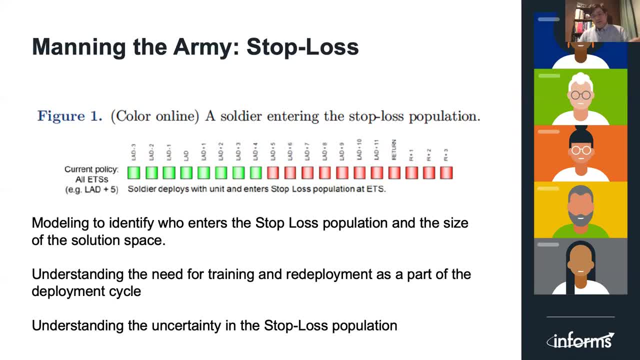 their tour and then translate or join the stop-loss population five months after they were in theater, And so really, when you're thinking about how we're going to deploy a soldier like this, there's really several different options. One would be well. 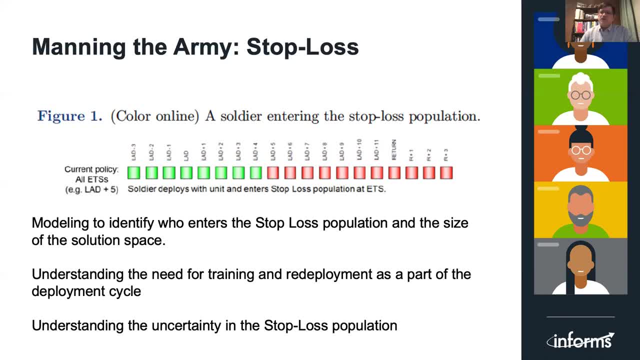 we don't know if this soldier is going to choose to get out of the army. so what we're going to do is we're just not going to deploy them at all. The other one would be: we don't care whether or not they want to get out of the army, we'll keep them until they redeploy and have them come as their. 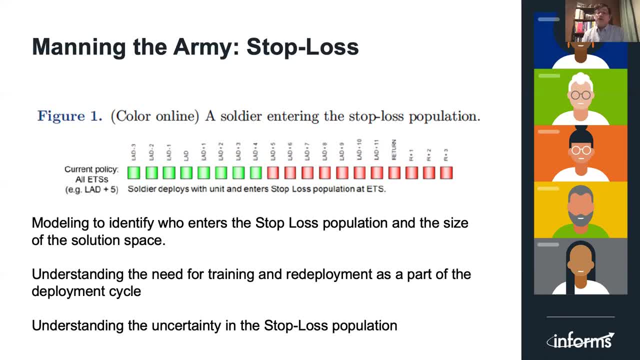 unit. And then there's the other decision, which would be well, whenever their time comes up, we'll send them home. But this kind of uncertainty where you don't actually know what the intention of the soldier is and you also don't know what's going to be happening in theater. 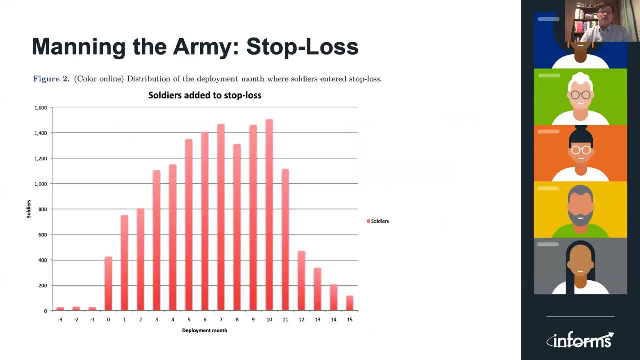 causes an interesting dilemma. And so, as you take a look at the number of soldiers that are added to the stop-loss population, you see how, over the number of deployment months, that the number of soldiers that get added to the stop-loss population keeps adding. Very few get added to the end as they're right about to come home. 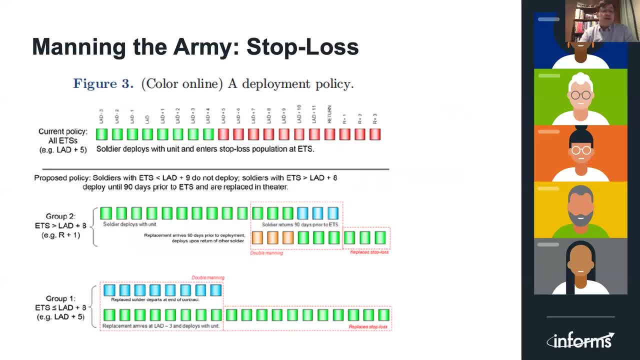 And so we take a look at how you man the army and you really have several different policies that you could imply And, as we take a look at when it became clear that we were going to stop doing stop-loss, then you have another decision which is saying: where are we going to double-fill? 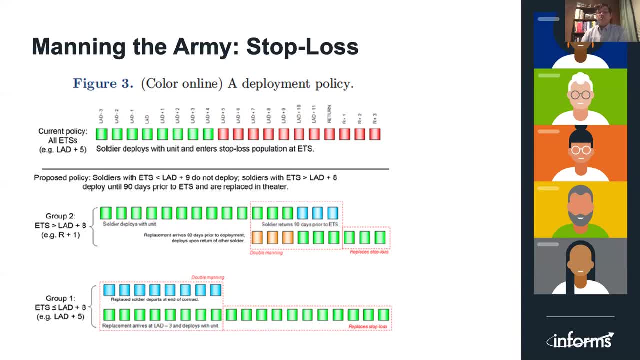 Or do we not send everybody that is going to? Do we leave during theater? Do we send them for half of their tour and then bring them back? When do we send the replacement? Because we're going to have to send a replacement And 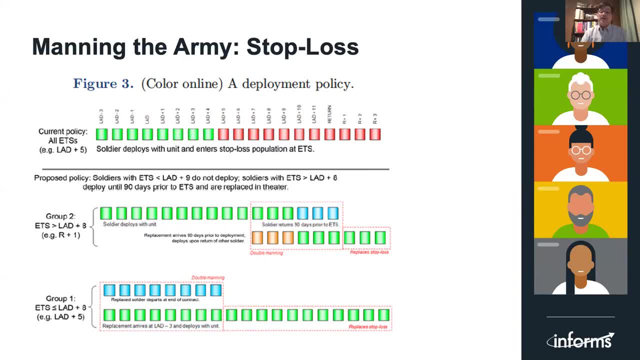 if you send a replacement four months before the end, you might have, as in the second from the bottom example, where you have the green chicklets represent the person that's actually filling the position You've got the orange one, which is another person that has been sent to prepare to. 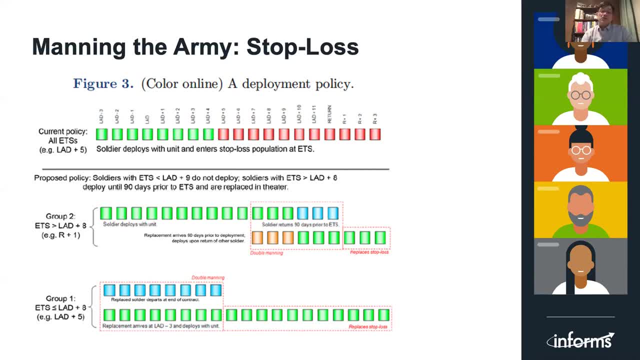 take over this position. And then you have the green one, which is another person that has been sent to prepare to take over this position. You've got the blue. as this green person transitions into redeploying- There's still a part of what we're paying for in the army, And so you have. 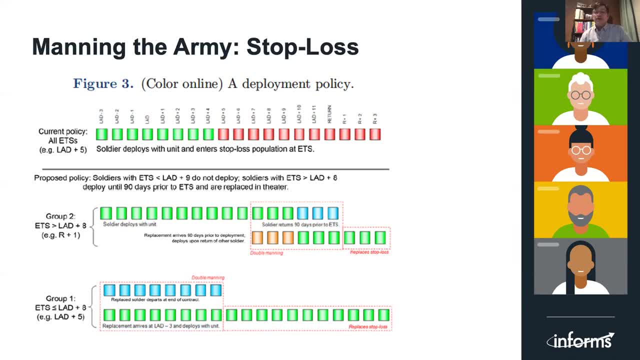 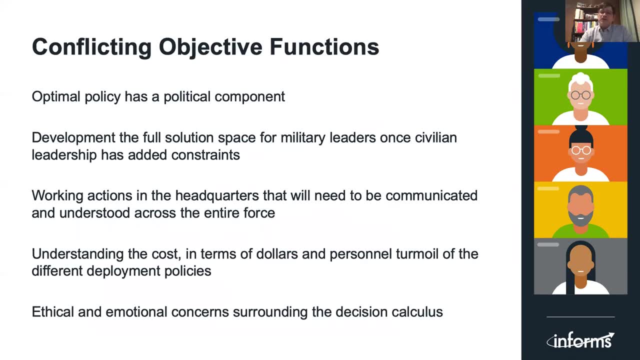 this point where you're paying for two people for one position, And so that really affects the readiness of our force. So one of the things that you really see here with this kind of a problem is the conflicting objective functions. An optimal policy has a political component. 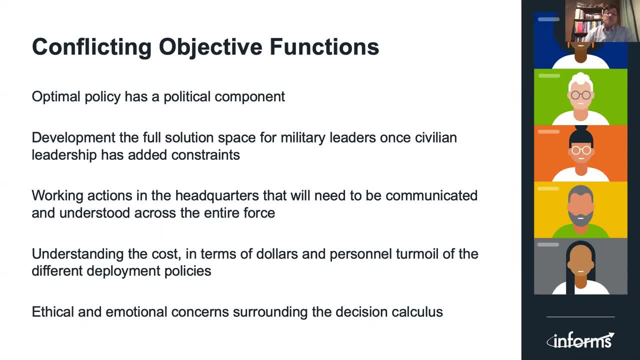 And, as you're really looking at developing the full solution space for the military leaders, often when a civilian leadership adds constraints, then you have a new area that you could possibly need to research for different solutions or find the most efficient solution within new constraints. 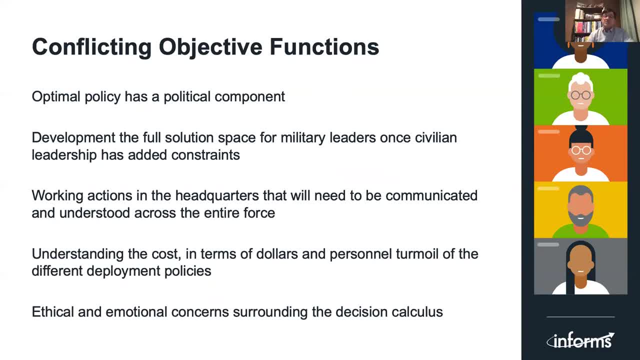 And this is one of those problems where you're working in the headquarters but the decisions that are made really have to be well communicated across the entire force And that, in order to suggest good problems or good solutions, you have to understand the cost in terms of dollars and personnel turmoil that will result from your different deployment policies. 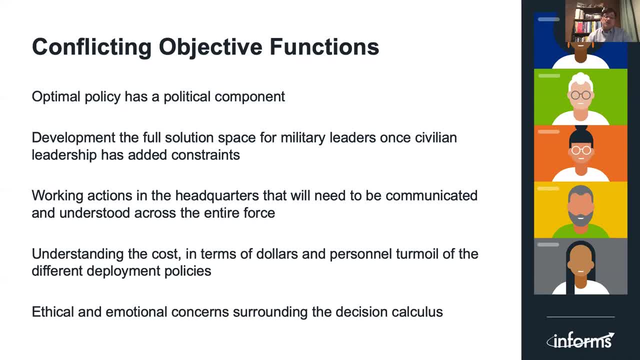 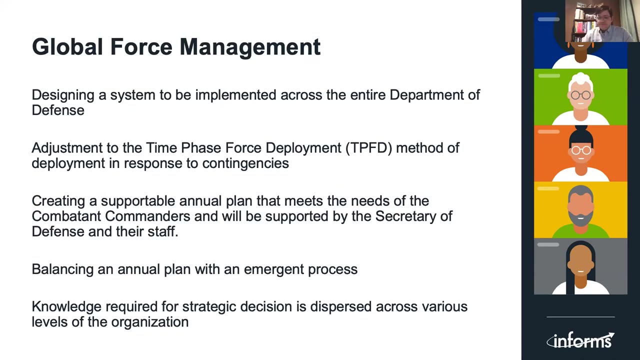 And also the ethical and emotional concerns surrounding the decision of when to deploy people, how to use a unit manning type methodology, but how much overmanning you need to accomplish to meet our objectives. So the last example that I'm going to provide is global force management, And this really 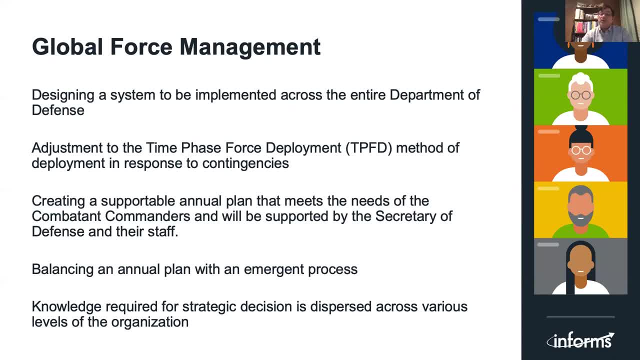 was a system where we need to create a new methodology for deploying forces in support of contingency operations. It used to be that all of our plans had a time-phase force deployment annex, which they still do, but that when they were doing something like invading Iraq, we figured they would just say: flow the TIPFID, send everything that we had. 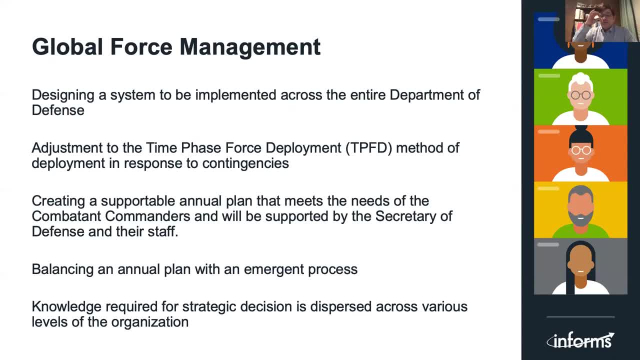 planned. But when Secretary Rumsfeld took a look, he said: well, I want to monitor, I want to meter the forces that are going into theater. And it really was when we started this notion of global force management And it's really creating a supportable annual plan. 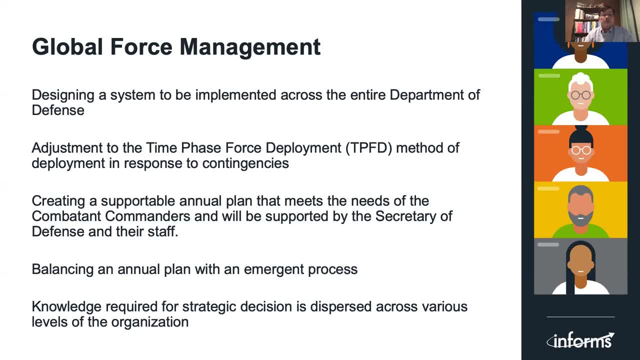 that will meet the needs of the combatant commanders, but also support the secretary of defense and the secretary of defense staff as being something that's aligned with our national strategy and balancing an annual plan with an emerging process, And it's one of the interesting problems. 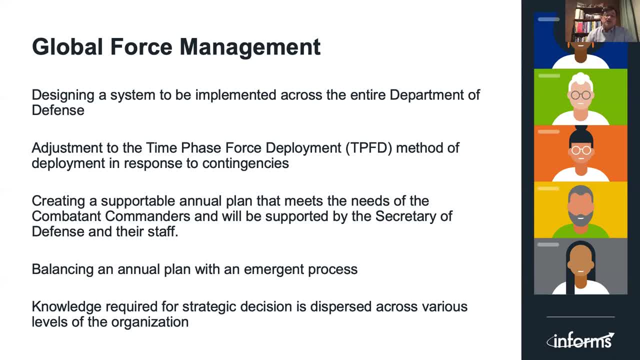 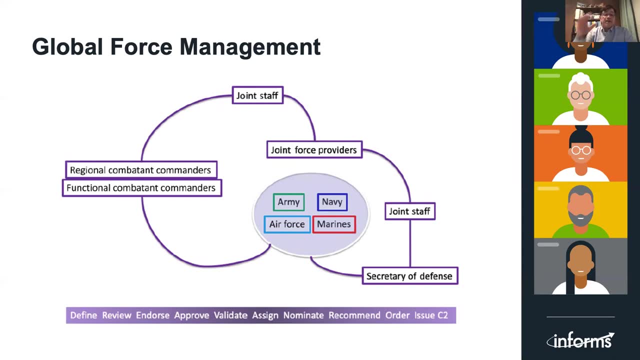 where the knowledge required for a strategic decision is dispersed across the various levels of the organization, Everything from the combatant commander's staff to the service staffs to the joint staff, where I was working. So the global force management process is one where we would define requirements. 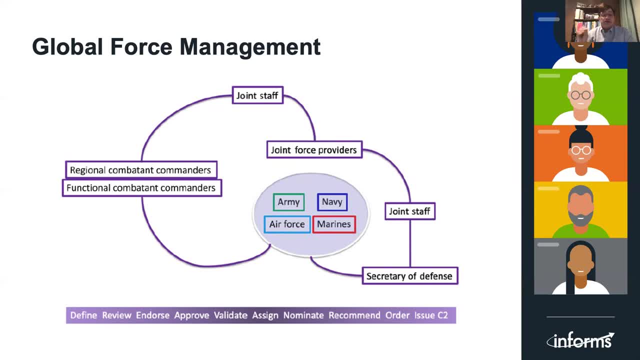 review requirements and you see across the bottom where we would endorse, approve, validate, assign, nominate, recommend order and then issue the orders. And so you have this cycle where the combatant commanders and the regional and functional commanders would come up with the requirements. 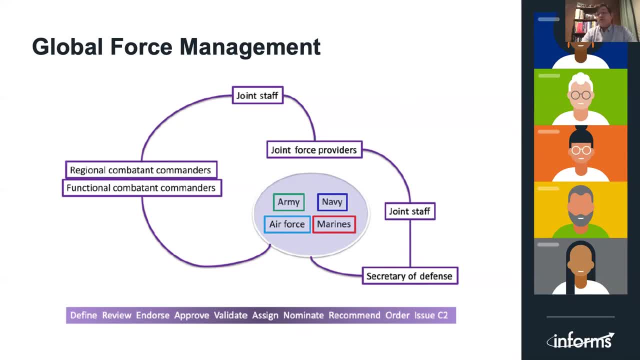 and they'd share this with the joint staff, who would then share it with the joint force providers, who would really find who was the best choice for this particular mission. They'd come back to the joint staff. the secretary of defense would order it. 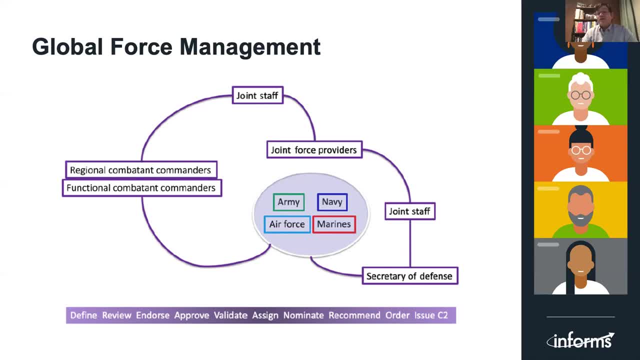 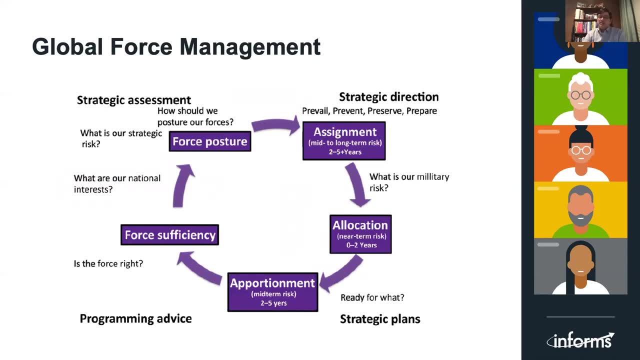 and then it goes back to the Army, Navy, Air Force and Marines for them to actually order the forces to move. But when we just take a look at a deployment order and come up with a whole list, a list of who we think we want to deploy, 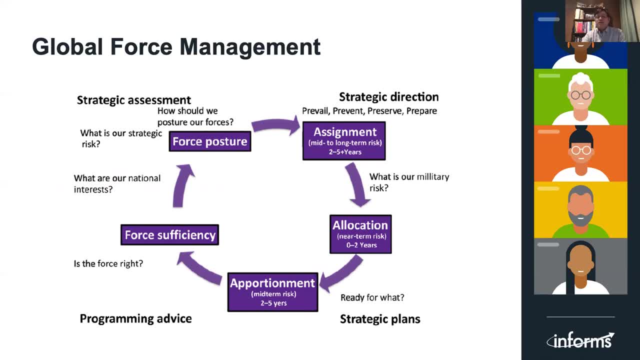 over the course of the year. it's not always clear why, strategically, we've made these choices, And so part of what we had to take a look at with global force management was really taking a look at the cycle of a strategic assessment. And you look at your force posture. 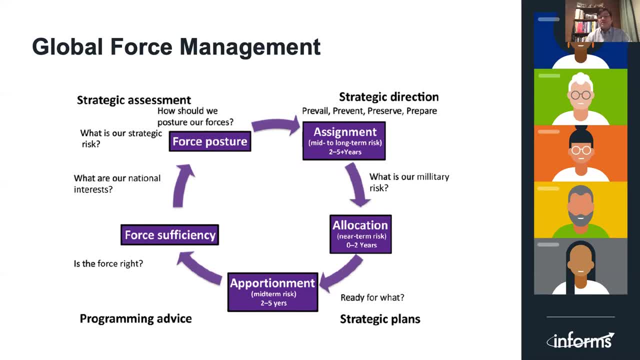 and you come up with an assignment of forces that's designed to place forces around the world in kind of a static location that we think makes sense. Then we use an allocation method to move people around as necessary, which is really in the short term. 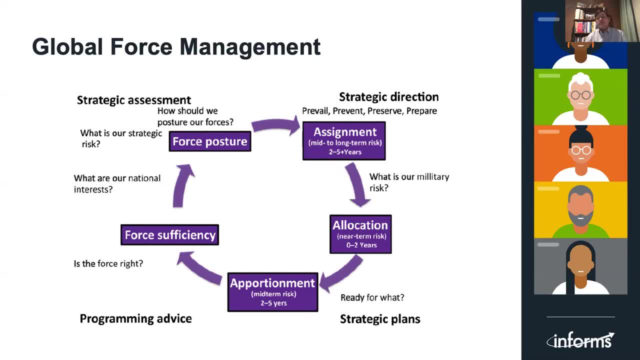 And we're constantly using an apportionment philosophy where you look at planning and you're saying who might we move? And when you take a look at who we might need, it goes back into the force sufficiency study to say: do we really have enough of the forces that we need? 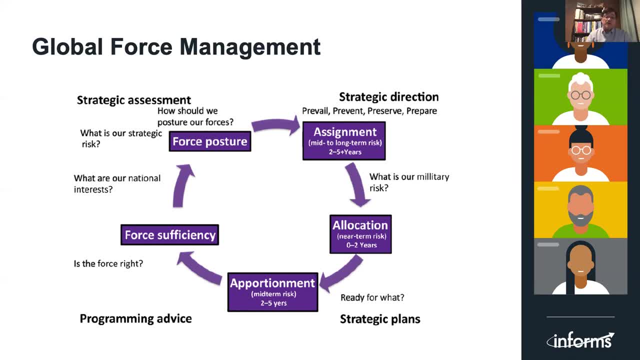 And then goes back into the force posture and the entire cycle it goes around, And so when you have this kind of a structure, it's easier for you to take a look at and explain to the strategic leaders the civilian leadership within the Pentagon. 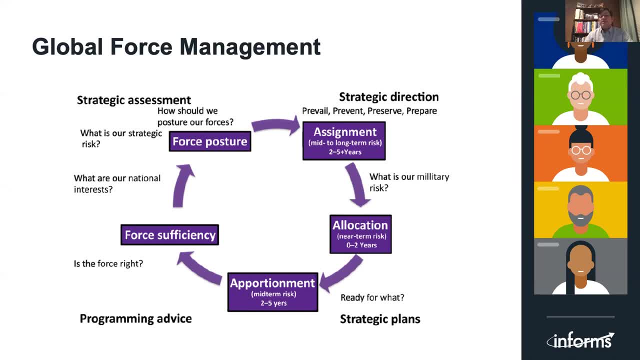 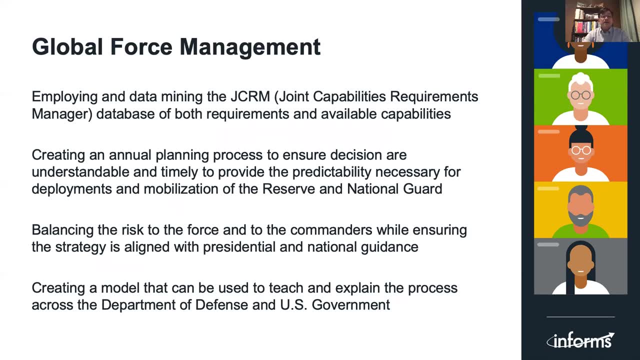 what were the planning assumptions that we used over the course of the year, And one of the things that we really had to come up with was a way to come up with the information about the data of what the requirements, what the requirements were, what the requirements would be. 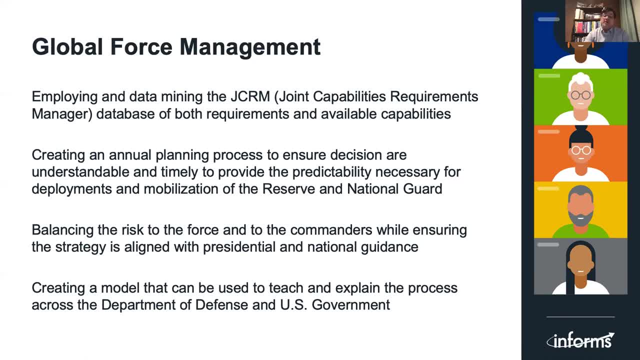 as well as what the forces available would be, And so we came up with a way, with means employing both: employing the J-CIRM data and data mining our J-CIRM data base, which really had both the requirements in it from the combatant commands. 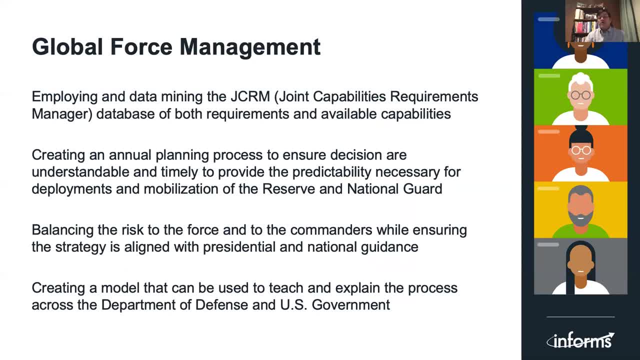 as well as the available capabilities, There was something that we could remotely use, and the combatant commanders were importing their requirements at the same time, the joint staff was validating them, And so it gave us a place that we would jointly work, but we also would be able to take snapshots out of that. 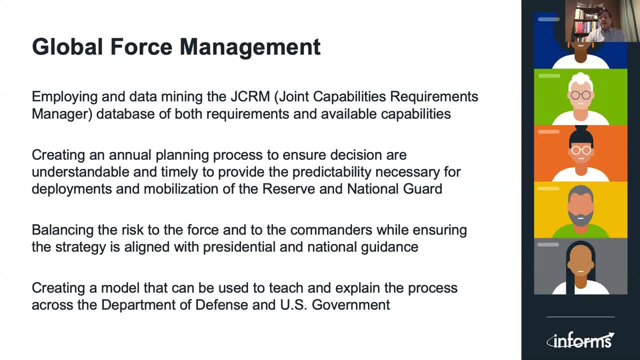 and data, mine that data to really figure out and to answer and create decision support. to explain what were our options when we were looking at the emergent opportunities, Because we would get a good plan in place but then there would be something around the world. 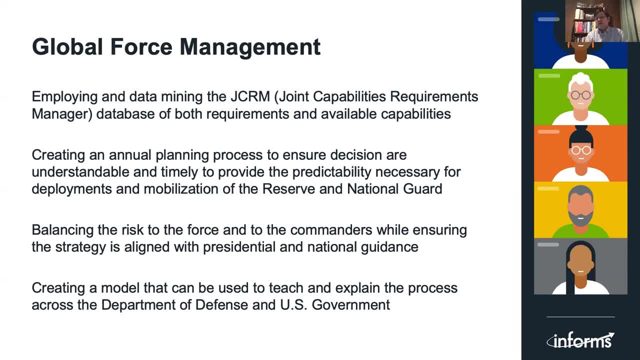 that would not be expected, And so you would use the data within the J-CIRM system to be able to see what were the upcoming requirements, what was our current force structure and really what we could change and look to order in the near term to solve some problems. 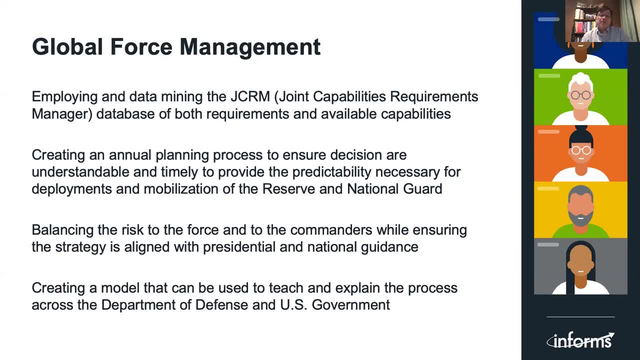 So we were creating an annual process that would ensure the decisions were understandable and timely, to provide the predictability necessary for our reserve and our National Guard, as well as our team members, Because we, as we, take a look at what we're building together, 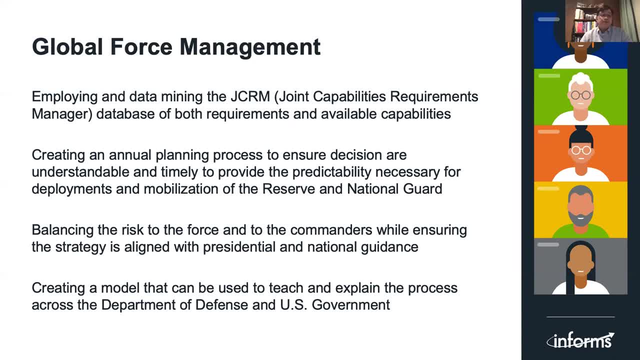 there's a certain amount of predictability that needs to go into to what we're doing, And we also were working on balancing the risk to the force and the risk to the commanders and ensuring that we were strategically aligned and being able to defend the strategic alignment that we had. 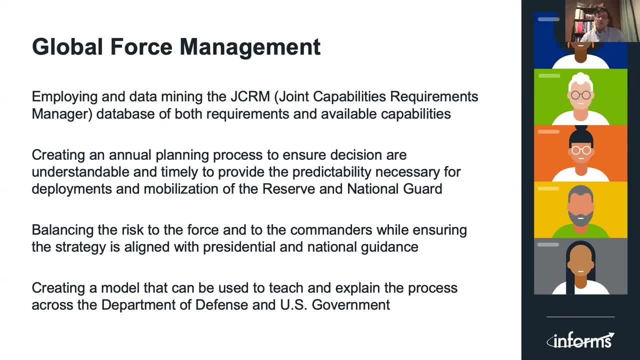 to the Secretary of Defense, And this is really an example where you know where you're creating a model that will. part of it is to teach the process to the people that join the team every year. Part of it is a way to explain our strategic thinking. 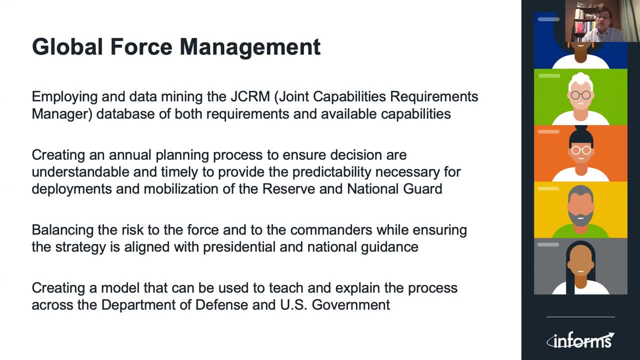 as we work together with our teammates across the Department of Defense, as well as the United States, the rest of the United States government, And it really was a great opportunity to work across the, in terms of you know, the entire joint force and was really quite an opportunity. 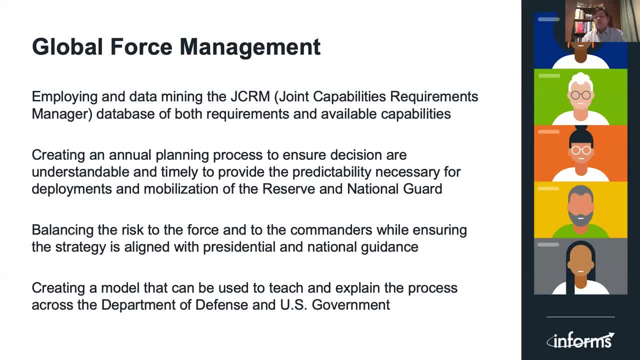 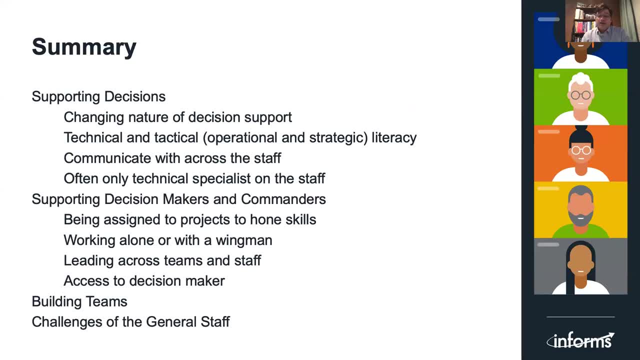 to create a new system and a new way of understanding what we were doing with global force management. So I'd like to close right now by looking at a couple of the ideas that we had here, And one of them is on supporting decisions, And so at the beginning, support might be talking. 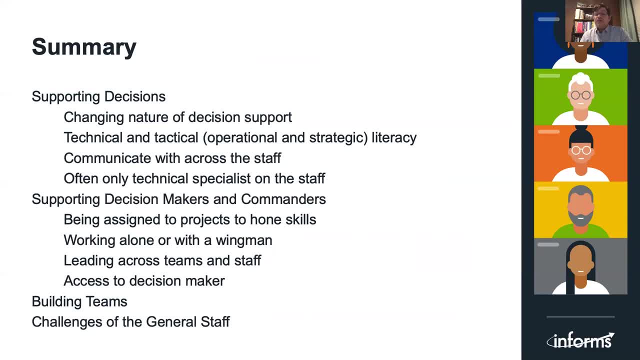 with your platoon sergeant underneath a pontoon right Or a macho with a red lens flashlight, And that's all the decisions before you get. But over time we really we have quite a bit of data and quite a bit of assistance that we can provide. 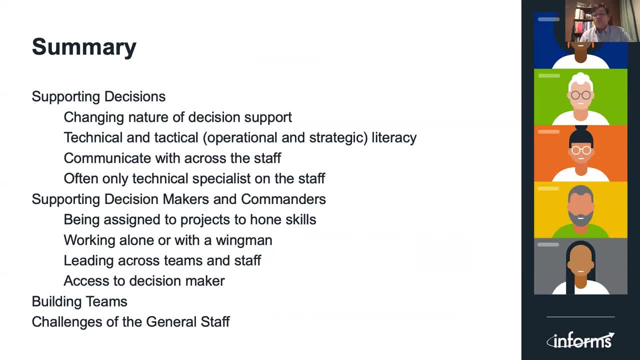 to our decision makers. But in order to be to really help in deciding these problems, you need to be technically competent as an ORSA, but also tactically And maybe tactically, maybe operational, but maybe strategic. But you have to have a literacy and domain knowledge. 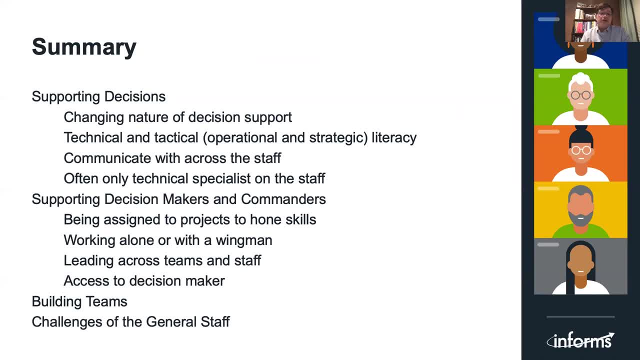 in what we're looking at, The software. Soft skills of working and communicating across the staff are crucial And, depending on where you are in your timeline, you may be the only technical specialist on the staff And you might have to be explaining to people. 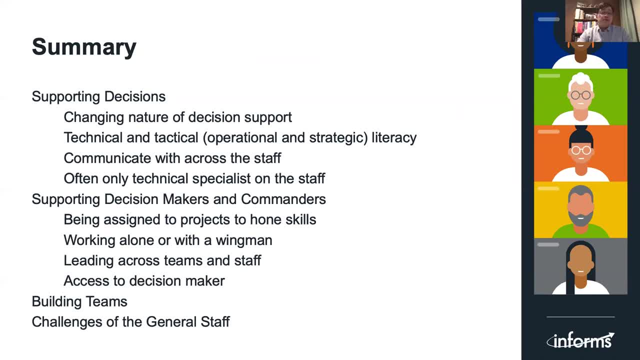 that don't understand your methods, why this method makes sense. So one of the things that we look at when you're supporting decision makers is: how do we assign people to positions so that they'll be able to hone their skills? How do you assign them to teams where there's a density? 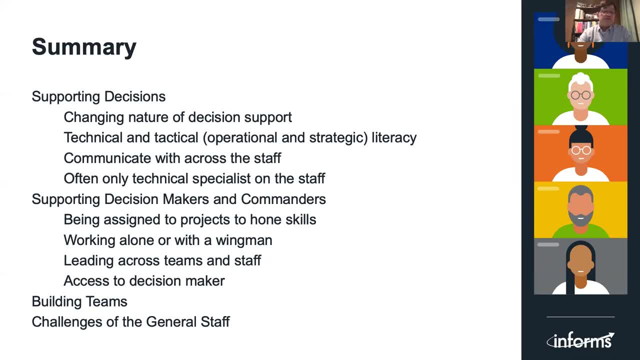 of ORSAs before you send them out somewhere by themselves. And you're going to have this opportunities to work by yourself, or maybe with just one wingman, And that is the kind of the second level after you've worked on teams. 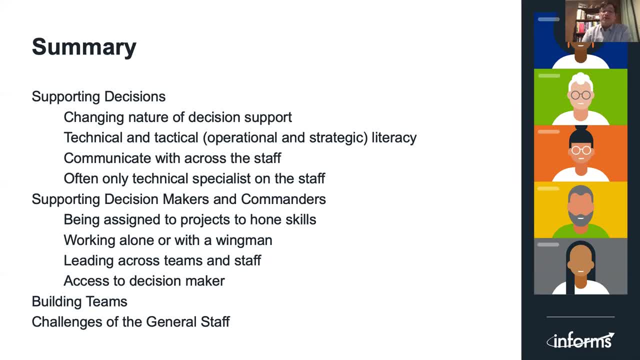 And then you really get to where you're going to be leading a team and working across entire staff sections where the ORSA support, or your teammates will really be in other organizations, And so you'll be working together on technical ideas, but you might have different assumptions based.